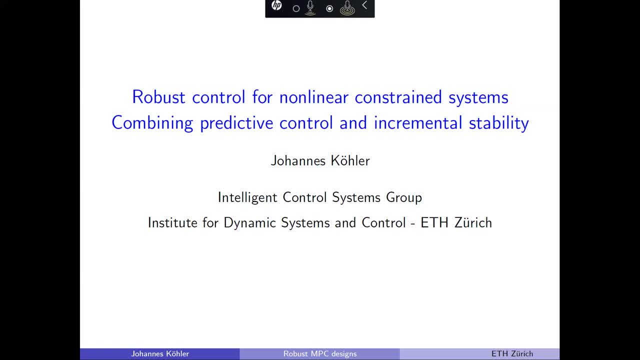 Welcome everybody to this week's Autonomy Talks. This week is a pleasure to have Johannes Köhler. He recently joined Professor Zeilinger's group as a postdoctoral researcher here at the Institute for Dynamic Systems and Control. Before that he received a bachelor's and master's in engineering. 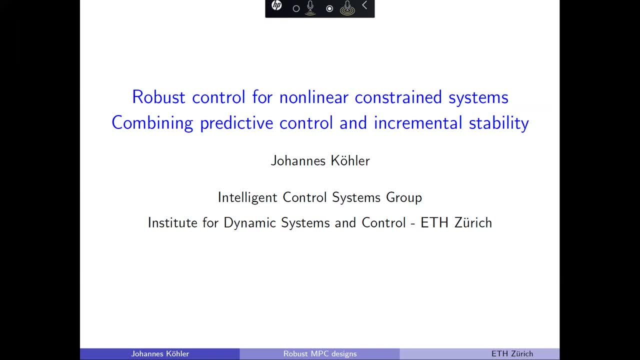 cybernetics from the University of Stuttgart in Germany, and he then did his PhD in the Institute for Systems Theory and Automatic Control, also in Stuttgart. His work focuses on non-linear and model predictive control. In particular, he focuses on the control of non-linear uncertain systems. 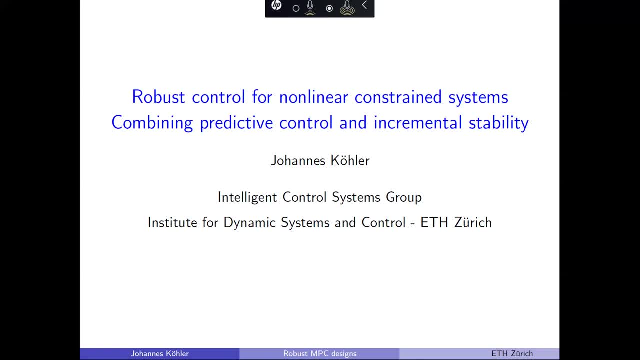 Today he's going to talk about some of his recent findings in these fields, and we're very happy to hear what he's going to tell us about. So go ahead, the stage is yours. Thanks for the introduction. So yeah, the talk will mainly be about how we 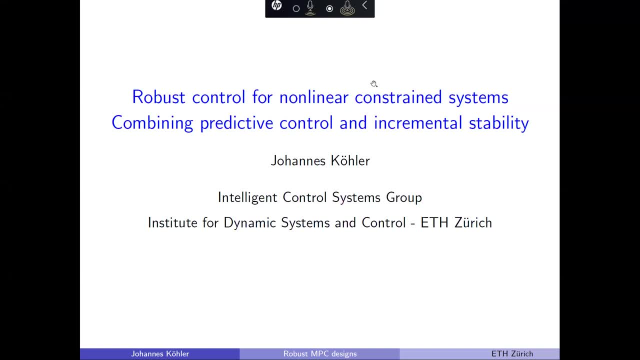 can look, if we have non-linear constraint systems, how we can ensure safety, critical constraint satisfaction, even in the presence of model uncertainty. And to do this we will mainly combine two complementary tools. One is predictive control, so optimization-based methods to handle non-linear constraint systems, And the other tool we'll use is incremental stability, which is a 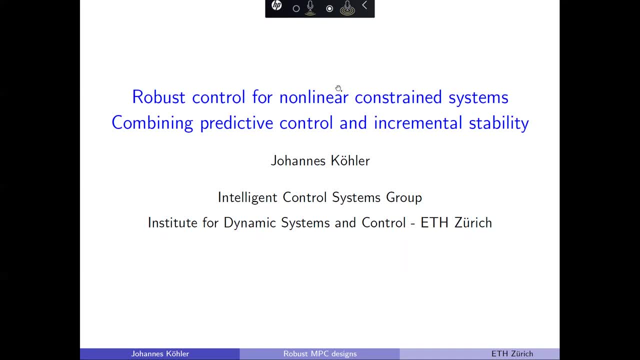 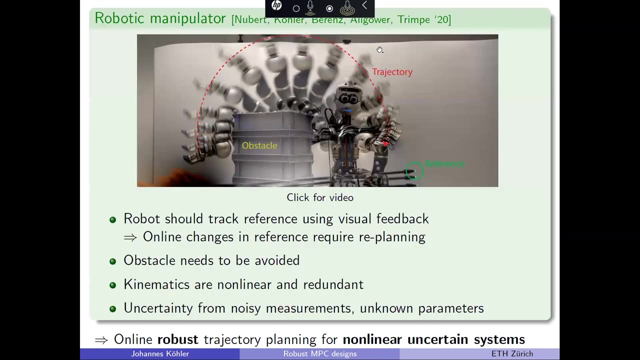 tool which can be used to analyze the robustness of non-linear systems And essentially, by combining those two different tools, we'll be able to handle non-linear robust systems even in the presence of constraints. Okay, first, as an example, to think about what other kind of problems we want to solve. 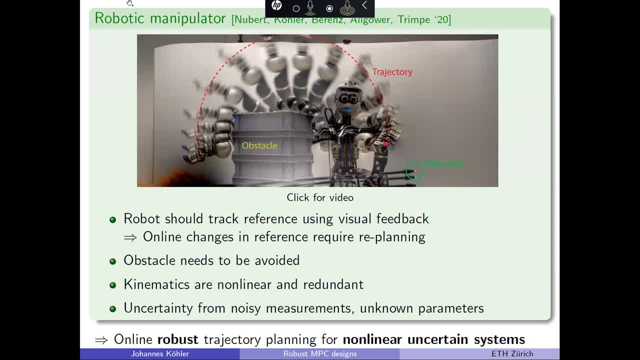 So this is the robotic manipulator taken from a recent collaboration I was involved in. We have here a robot arm Over all the kinematics and dynamics of this robot are non-linear and we have here a reference which is measured with motion capture And the robot wants to track this reference with this arm. 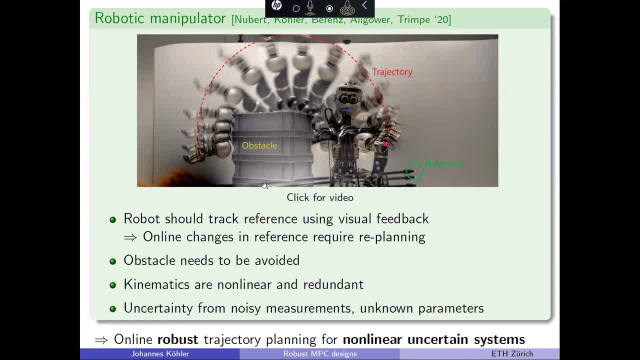 while also avoiding some obstacles. And furthermore, in the overall setting, we have various sources of model uncertainty, like measurement, noise, parametric errors. So what actually needs to be done to make this whole thing work is that, online, if we get a new goal where the robot has to go, we need to be able to. 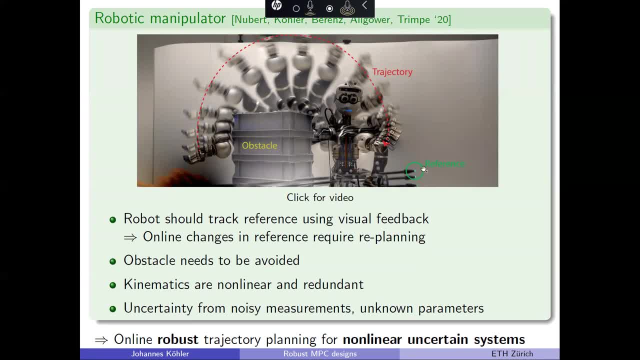 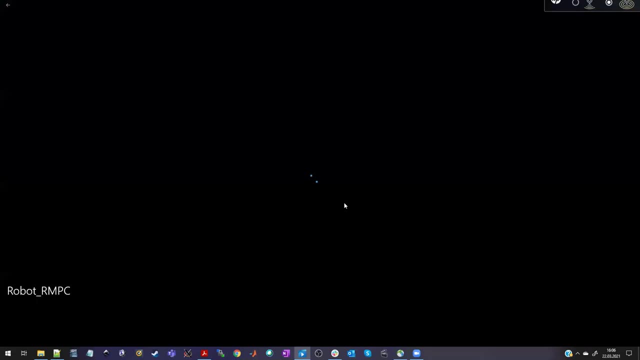 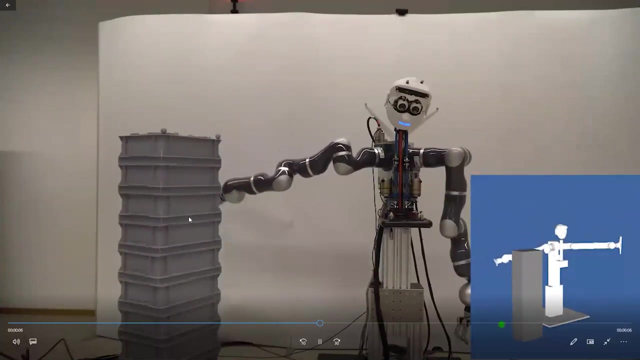 plan a trajectory to reach our target in a reasonable time online. that also guarantees that we can avoid those obstacles robustly, even though we have model mismatch. and maybe to give you an idea how this looks, it's a very brief video so you can see here there's a motion capture and if the target is behind obstacle, that he 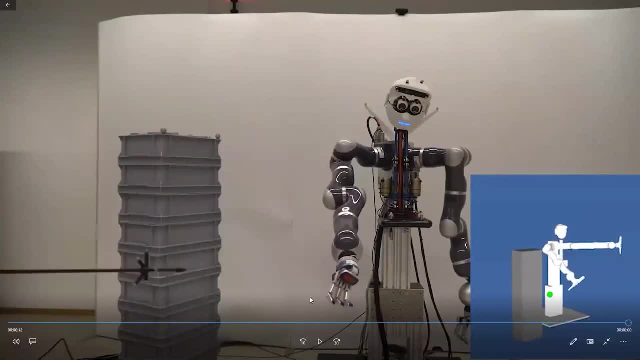 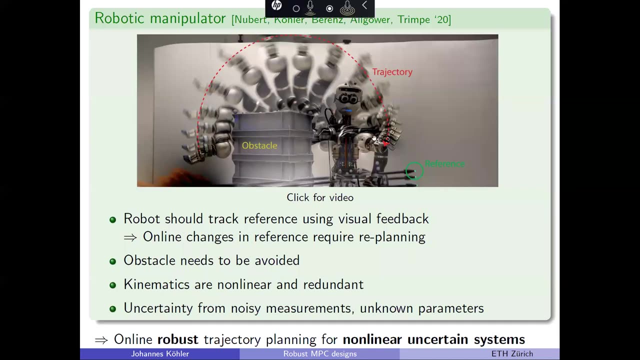 can't reach it, he will stay always safe, but then he will always try to find a way around the obstacles to kind of achieve this goal, and so what we need for those kind of problems are essentially online, robust, objective planning methods which are applicable to non-linear 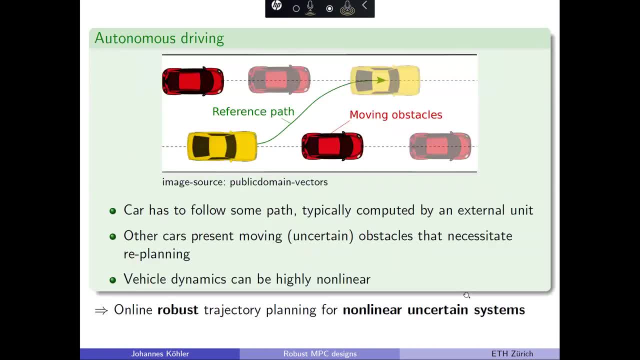 and uncertain systems and similar problems also appear if we think of autonomous driving or maybe cryptocopters- that essentially we need to. we often have non-linear systems. there are various sources of motion capture that are in the way of non-linear systems that are very similar to what we're seeing. 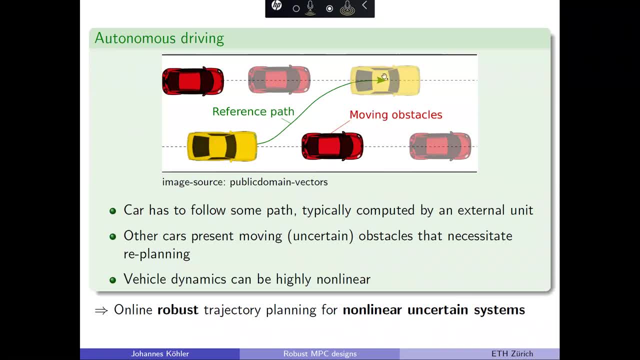 in the future of non-linear systems. they're very similar to what we're seeing in the future of model uncertainty. we often have to plan paths online which avoid different obstacles, and often we have to do online replanning, and that in a robust fashion, yeah, and so, to summarize what? 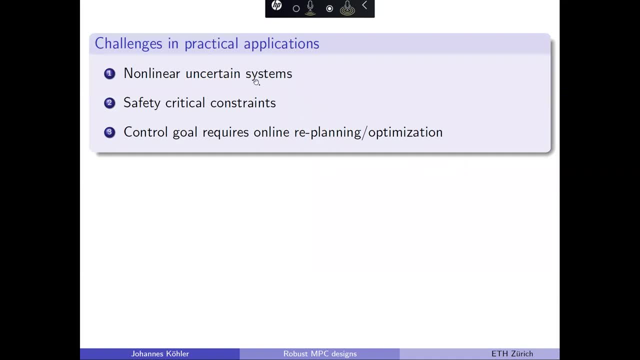 you basically need. so the challenges you have are: you have non-linear, uncertain systems, you have safety critical constraints that you want to meet and typically you also have some kind of control goals which require online optimization and replanning in real time and, as i already mentioned, we'll combine two methods to deal with this. 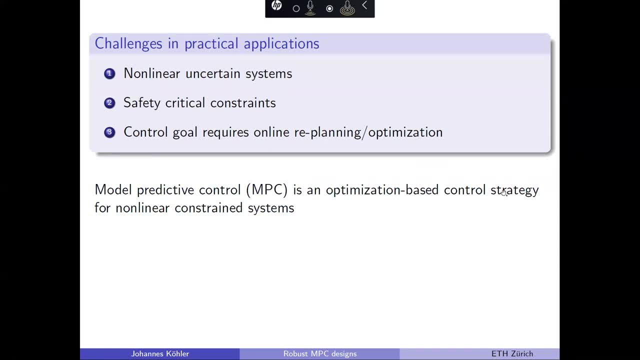 one is model cryptic control, which is an optimization based control strategy which is applicable to non-linear constraint systems, and the other tool is incremental stability, which can be used to study the robustness of non-linear controllers around arbitrary trajectories. and, in a nutshell, you can use this to study the robustness of non-linear controllers around arbitrary 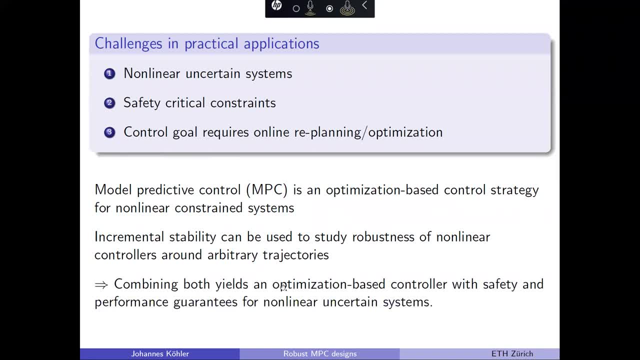 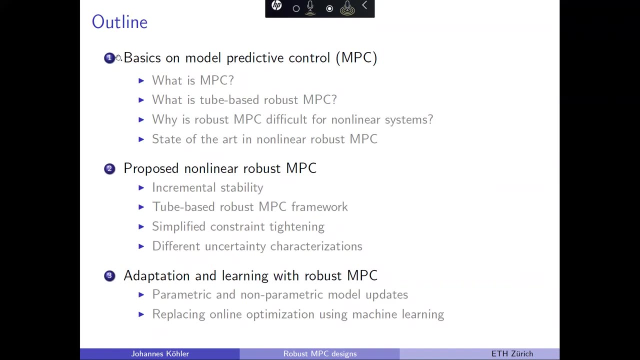 trajectories and, in a nutshell, you can use this to study the robustness of non-linear. by combining those two different methods, we'll be able to get an optimization based controller with safety and performance guarantees for non-linear and uncertain systems. okay, so briefly, how's this talk structured? first, i'll introduce some basics regarding 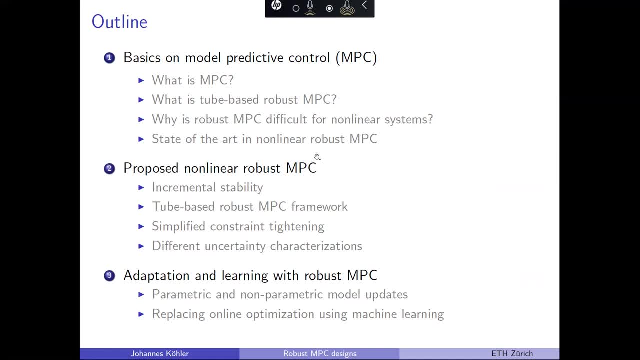 model predictive control, then i'll present a proposed non-linear, robust npc framework and they and i'll briefly talk about adaptation learning- how this can be used to further enhance performance. so first, very briefly, i'll talk about more predictive control. what is one predictive control? what's robust npc? why is robust directive control difficult for non-linear systems? 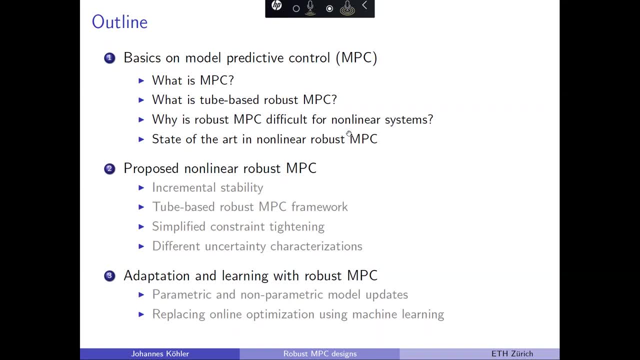 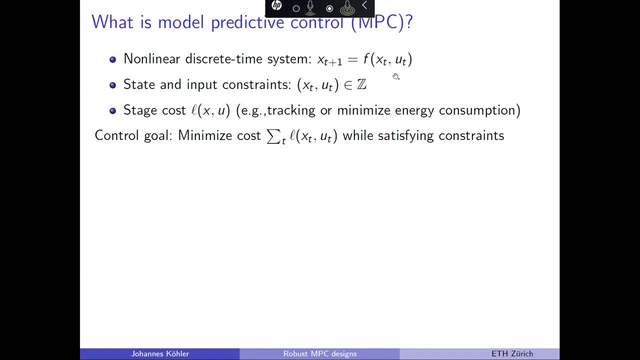 and what's the state of the art to do this for non-linear systems? okay, so what we look at in only a more productive control are typically general, non-linear, discrete time systems. we can also look at continuous time systems And, what's important, we are able to consider general state input constraints. so both actuator 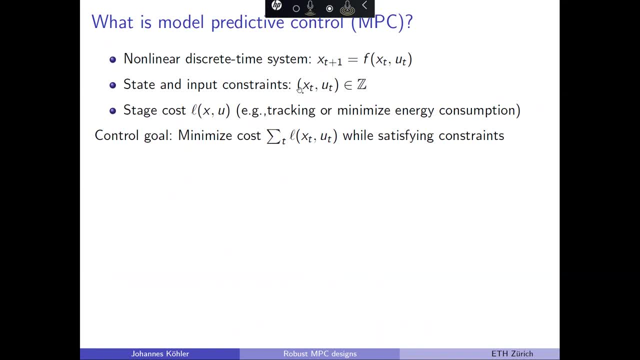 limitations and safety-critical collision avoidance constraints, And typically we also have some kind of stage cost or reward function that characterizes our goal- So, for example, tracking a goal or minimizing energy consumption- And so the overall goal that we want to achieve is to minimize this running cost, while also 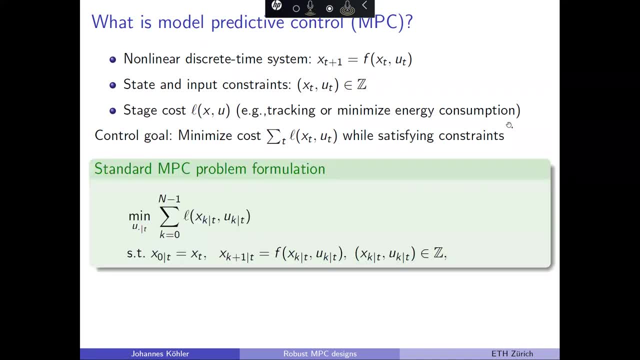 satisfying our constraints. And a prototypical MPC formulation looks as follows: Given a measured state, we optimize our finite horizon input sequence, predict a corresponding state sequence, Then we make sure that the resulting state input sequence satisfy the constraints And then we also minimize the finite horizon cost function given by some of stage costs. 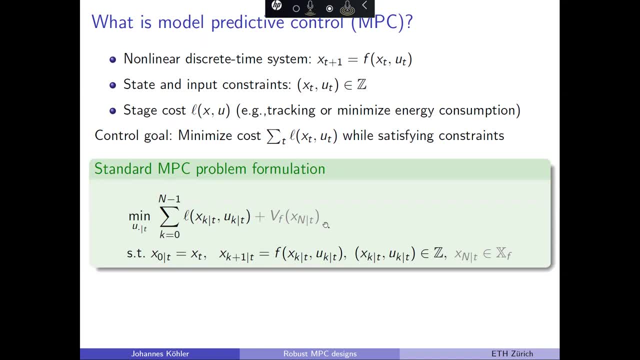 Now, depending on the formulation, you might also have an additional cost and a term set constraint, But in this presentation I will simply ignore this issue. but this can also be handled. And now, what you actually do in closed loop in MPC is: in every time step you measure. 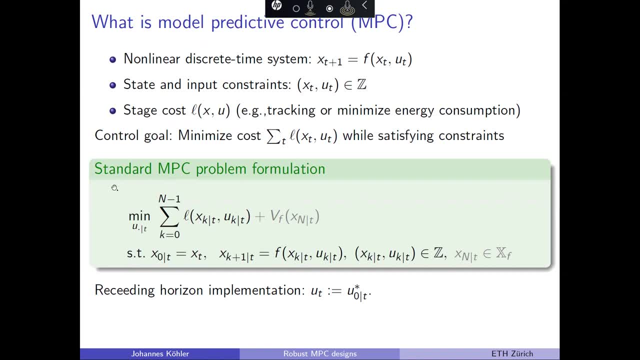 your state. You solve this finite horizon open loop optimal control problem, which is a nonlinear program, And then you get an optimal open loop input sequence and you only apply the first initial part of this input sequence to your system. Then you remeasure your state at the next time step. 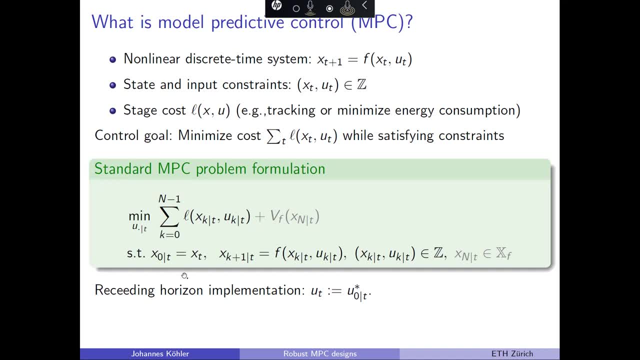 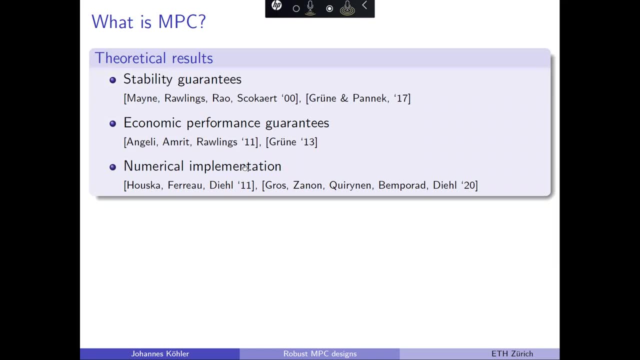 And then you repeat the whole procedure in a receding horizon fashion. So MPC is a rather not new technology or recent technology, but still there are a lot of established results for it. So it's well known how to guarantee stability, how to also provide performance guarantees. 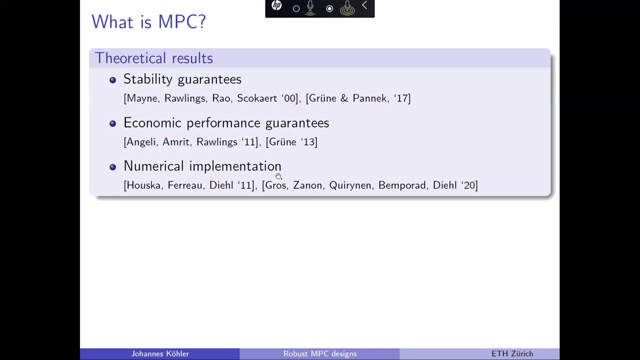 if you're not interested directly in stability, And there are also a lot of efficient numerical implementations such that you can really bring it down to real time. But what is a little bit lacking in a lot of those theoretical results, It's that most results assume that the model is exact, and this is of course, already. 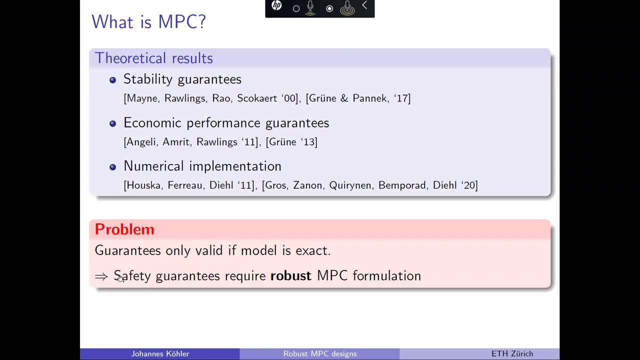 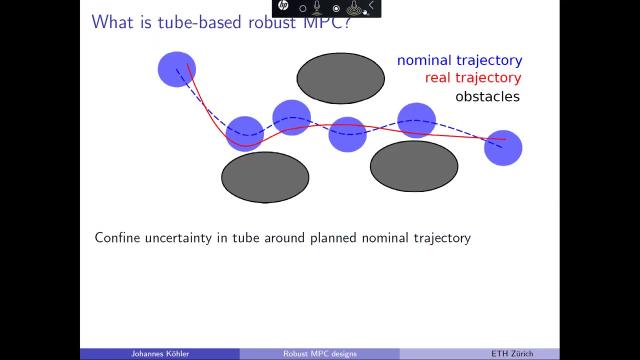 the case in practice, And especially if we have safety-critical hard state constraints, we really need to modify the MPC formulation to be robust and to take uncertainty into account. Now, one way to take uncertainty into account is shoe-based, robust MPC, which is one of 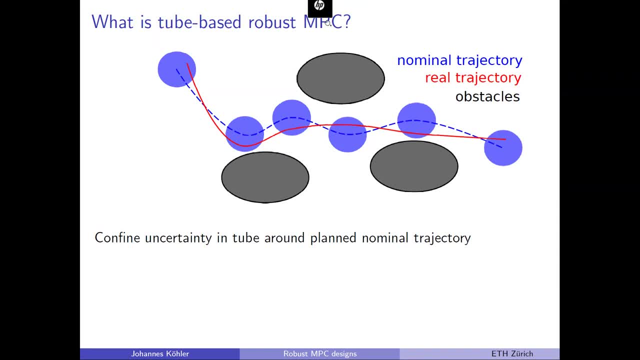 the simplest and, I would say, most popular approaches. So let's take a look. The idea is rather simple. We have some uncertain state prediction here in red which we don't know exactly, And since it's difficult to do predictions with this, we instead use a nominal prediction. 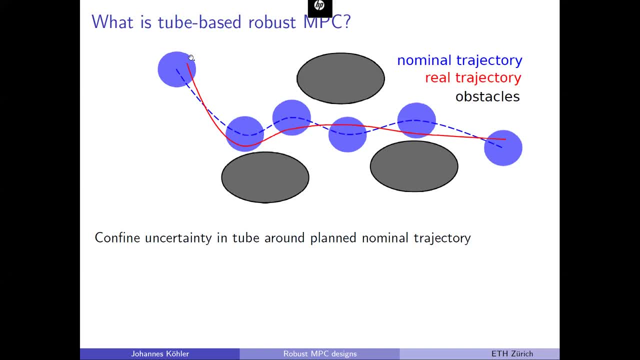 here in blue and then compute a cube or funnel around this trajectory here given by those blue circles, And then we want to make sure that the uncertain system with disturbances will stay close to our nominal trajectories in those cubes. If we can somehow guarantee this, then we can simply plan with a nominal trajectory and this additional 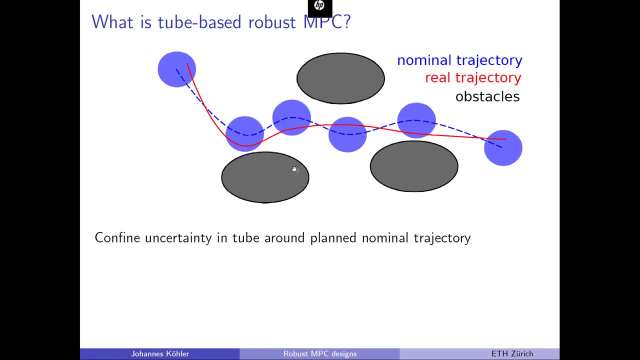 cube around it and make sure that this cube avoids the obstacles robustly, And then we can be sure that also this uncertain trajectory will be safe. So really the idea is to plan nominal trajectories and put a cube around those nominal trajectories where the uncertain system should be contained. 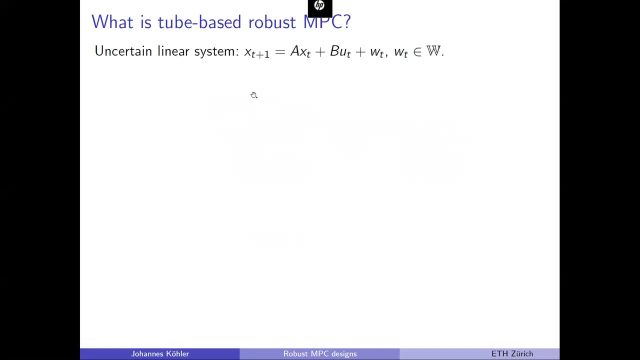 Now for LIA systems. it's actually quite easy to do So. if you have a linear, discrete time system with some additive disturbances, W which are unknown but bounded, then there's a classical solution to this by Maynard from 2005,, where 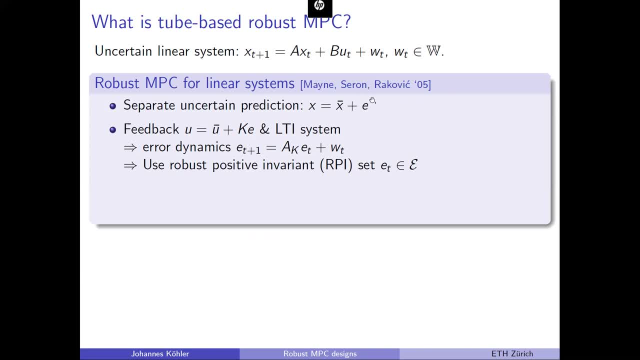 you split your uncertain state predictions into a nominal prediction and an error. If you then use an additional error feedback that you apply to your system and you use the fact that you actually have a linear time invariant system, you can show that the error dynamics behaves according to this simple linear map. 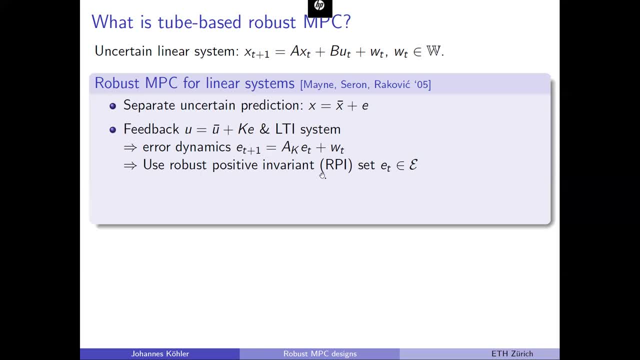 Okay, For this linear system. you can then compute a robust positive invariant set where the error is contained for all time steps. Now, if you've done this offline, online you can simply plan a nominal trajectory with a tightened constraint set depending on the magnitude of this RPI set. 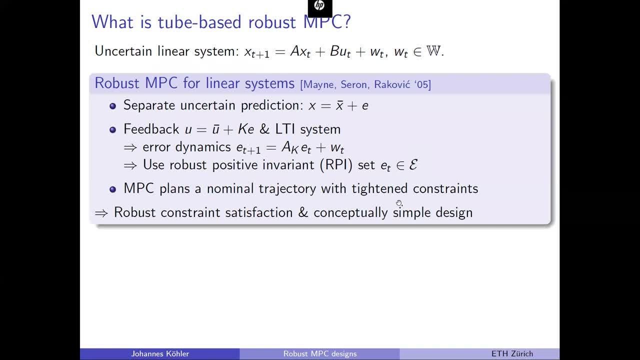 So it's a rather conceptually simple design, easy to apply, and you get your robust constraints, satisfaction guarantees and similarly also performance and stability. Now, what's the limitation Is, as soon as you go from LTI systems to nonlinear systems, you cannot separate those error dynamics. 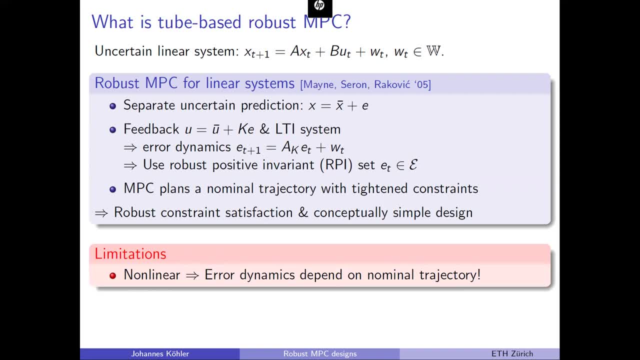 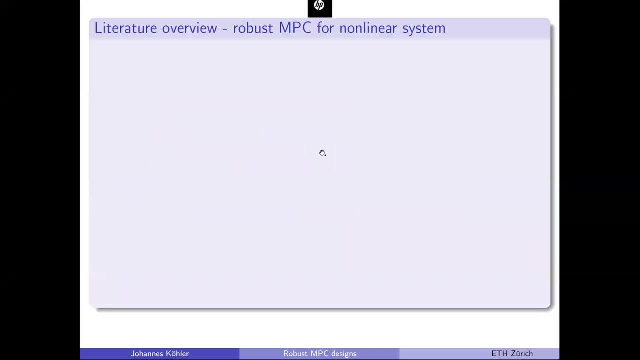 So you will find out that actually how the error evolves into the future also depends on your nominal trajectory, because the system is nonlinear And this makes this whole idea of computing RPI sets non-trivial. Because of this, there have been a lot of different approaches in literature how to 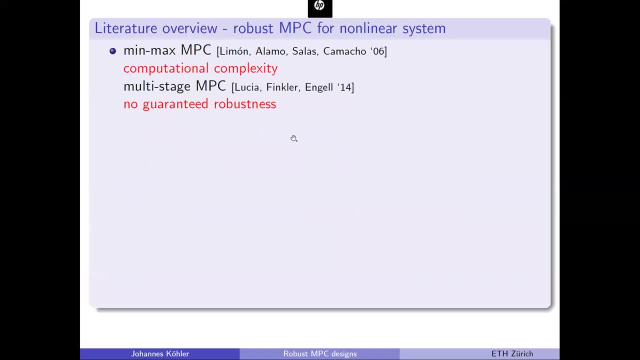 deal with nonlinear systems. So let's take a look now at some of the other approaches for working with rally and inflation systems. So here on the left, here you can see that the RCR, or the game model, is a representation of the risk and uncertainty. 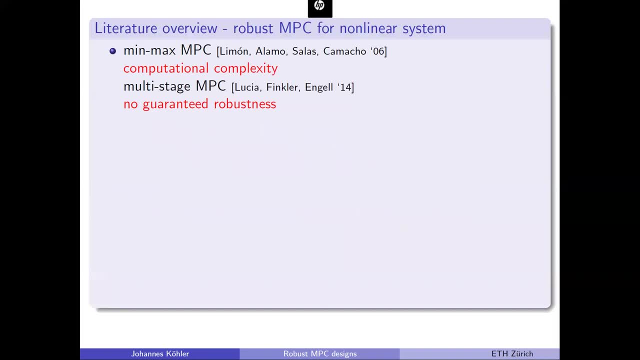 Rather classical ideas are min-max MPC schemes where you online optimize a kind of worst case disturbance. Now this is quite nice, but it actually can be very computationally complex. There are also approximation stuff like multi-stage MPC, but then you typically lose. 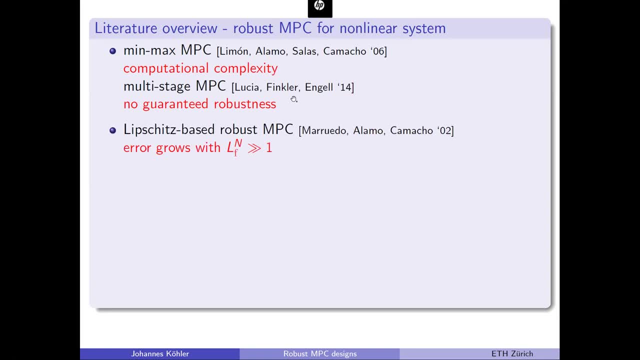 your vertical guarantees. There are also, on the other spectrum, rather simple methods where you just use, for example, Lipschitz concept of your system to provide an over approximation of how you generate a impact, Like if you use a R Mazda here. 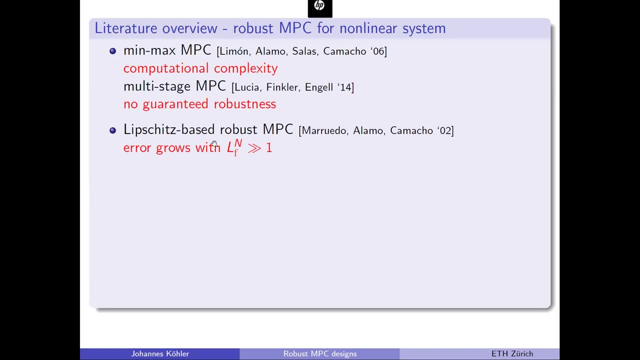 See the R Mazda. we have one on the left side which is kind of a very powerful method, the of how the uncertainty propagates over your system. but then your predictions of your arrow grow with the Lipschitz constant to the power of the prediction horizon. 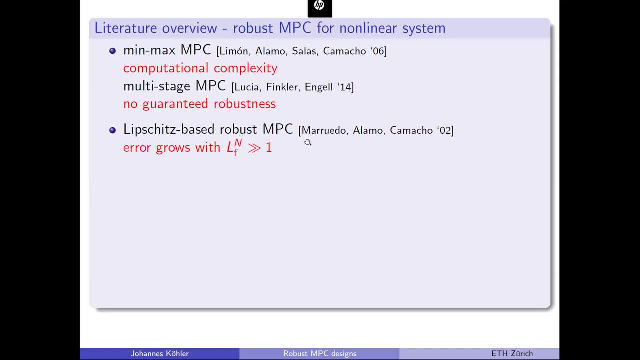 and this can be very conservative, So it's often difficult to apply for long horizons. More recent ideas are also max differential inequalities. There you kind of online optimize those ellipsoidal sets and this gives you a lot more flexibility. but this also means you have to online optimize. 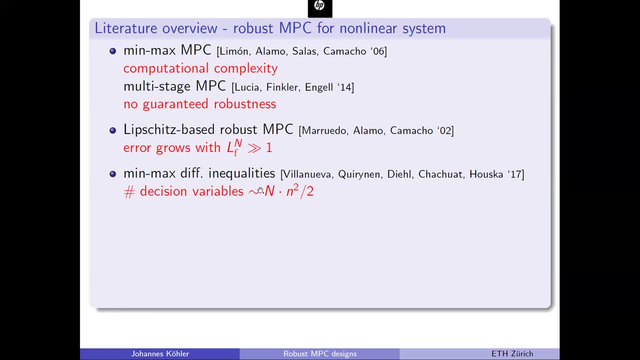 over ellipsoidal sets and this increases the number of decision variables drastically, particularly quadratically in the state Last. there are also ideas to kind of try to stick to this idea of RPI sets and extended nonlinear systems using tools like incremental stability. 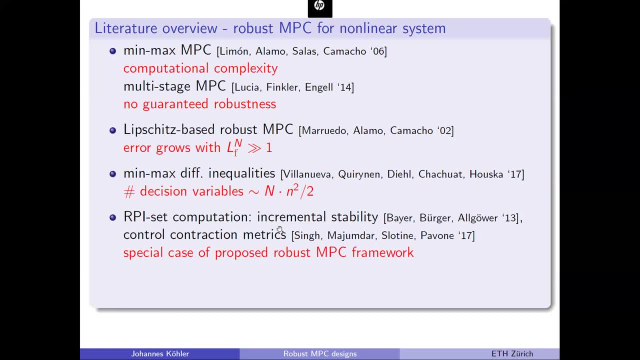 and control contraction matrices, and we'll see later in the talk that those are particular special cases of the proposed robust MPC framework. And lastly, what I also mentioned are also ideas, not too much from the MPC community but more from robotics communities. 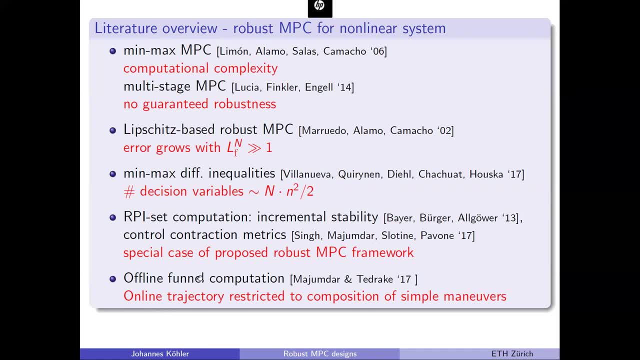 for example, based on funnel computations, maybe for a specific trajectory you would be able to compute a good tube, and if you can do this for a lot of trajectories offline, then online you can simply put together your trajectory as a composition of simple maneuvers. 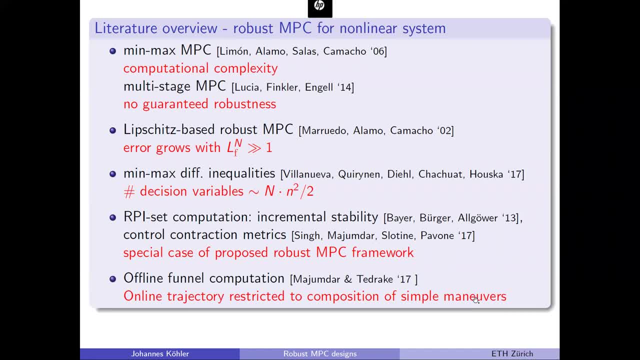 The problem is, of course, this is only applicable if you can actually- if it's meaningful to online- compose your real trajectory based on you know. if you can actually- if it's meaningful to online- compose your real trajectory based on simple maneuvers. 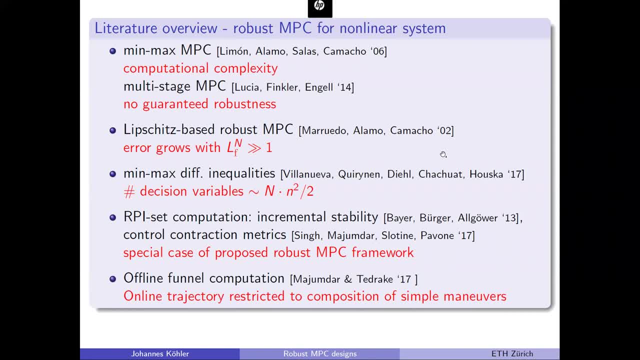 and depends a little bit on the application. Okay, so this is what exists, and the goal now in this talk is to provide a more general framework: how to do nonlinear, robust MPC design, in particular, both those simple Lipschitz-based approaches. 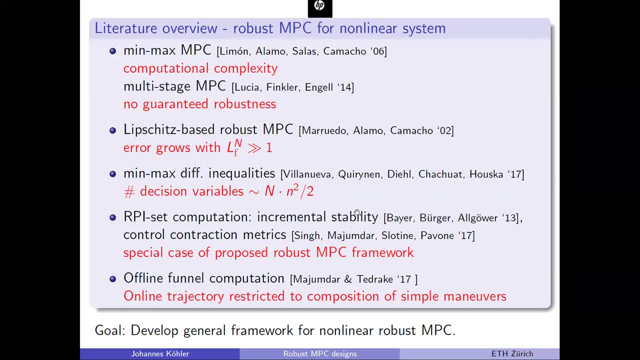 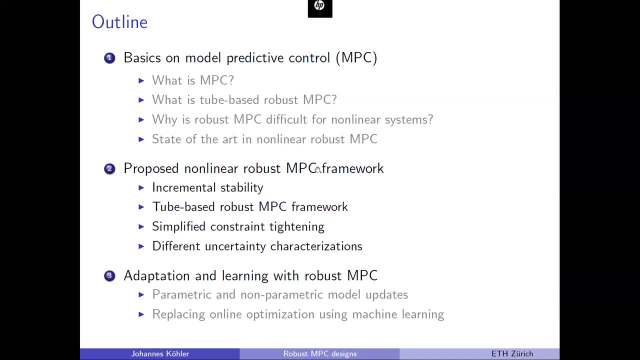 and those ideas based on RPI sets will be contained as a rather simple special case of this framework. Okay so, given this brief overview, Okay so, given this brief overview, I'll next present a proposed framework where I'll first introduce the notion of incremental stability. 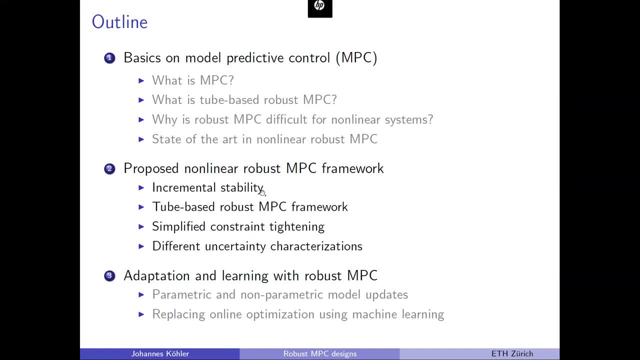 and this will be the backbone of the proposed formulation. Then I'll present the proposed framework- a simplified constraint tightening, which is very important for efficient numerical implementation, and then I'll also briefly talk about different uncertainty characterizations. Okay, so, like I said, 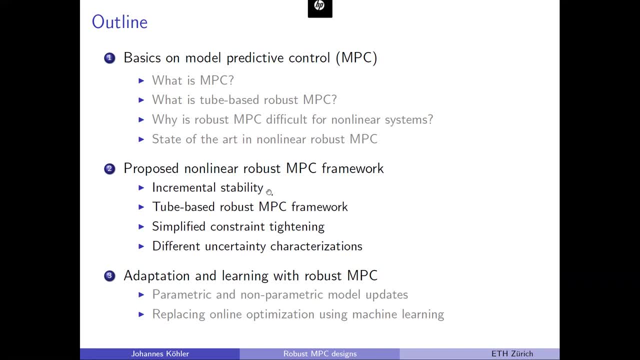 I'll first talk about incremental stability and this system property will be- they'll be the basis for this. Okay, so, like I said, I'll first talk about incremental stability and this system property will be- they'll be the basis for this. 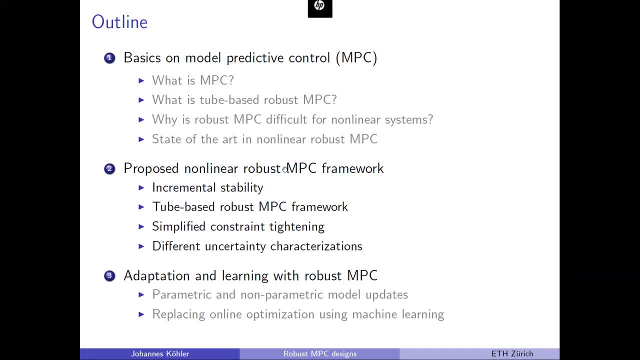 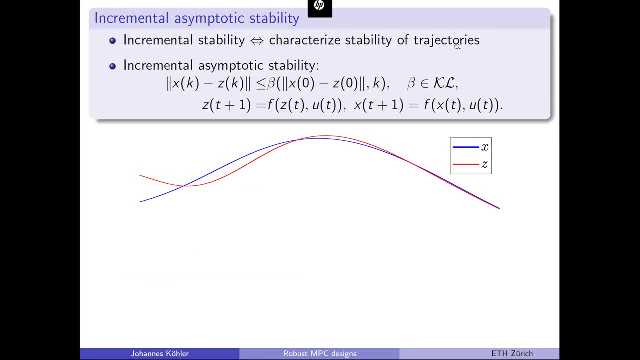 and this system property will be, they'll be the basis for this nonlinear uncertainty propagation, nonlinear uncertainty propagation. So what is incremental stability? Essentially, this is a property that characterizes the stability of trajectories. So, more formally, a system is incrementally, asymptotically stable. 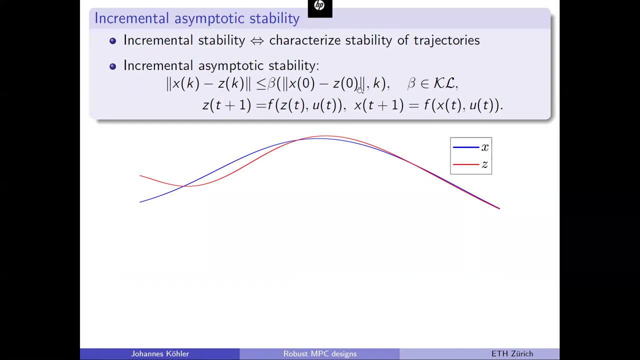 if we have two systems with the same dynamics, two different initial condition, and they converge to each other. So, in a picture, if I have one trajectory and I have another initial condition and those two trajectories converge to each other, the system is incrementally stable. This property can also be equivalently characterized using Lyapunov. 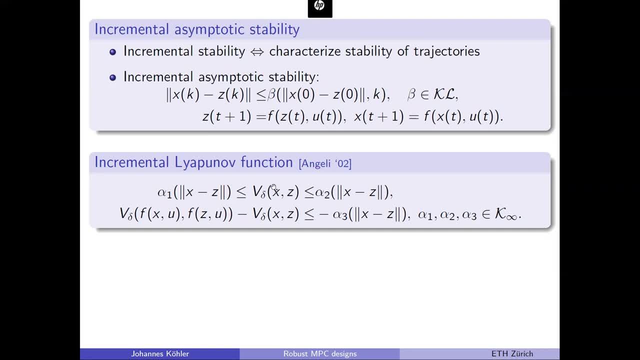 functions that are called incremental Lyapunov functions, which is a function of both of two states because it measures the stability of two trajectories, but similar to the standard Lyapunov function. it's lower upper bounded by the distance of those two states and it's somehow decreasing. 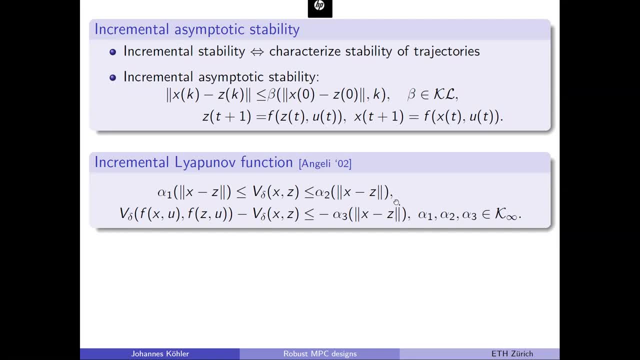 by the distance of those two states. To make our life simpler, we can also consider exponential decay, Lyapunov functions, and this just means, instead of a channel decrease, we assume that we have an exponential decay, which makes the exposition a lot easier. and here we have some. 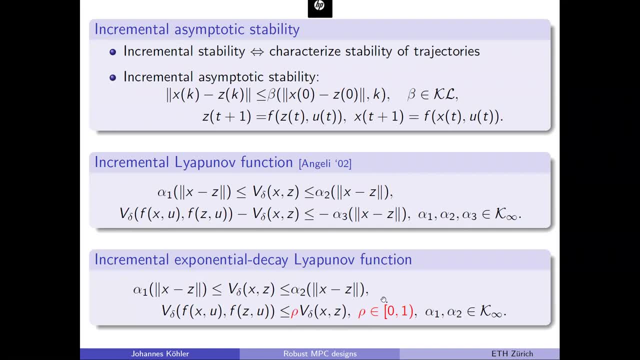 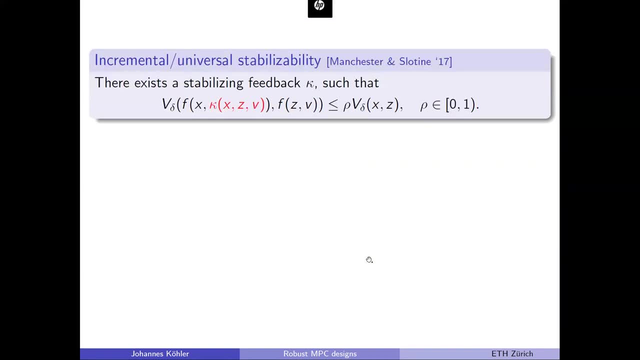 contraction rate rho smaller one, and we'll see later how this is important for the formulation. Actually, assuming stability is restrictive. so what you do in this case is that you have a constant decay and you have an exponential decay, and you have a constant decay. so what you do instead is you actually assume stabilizability. so this is called. 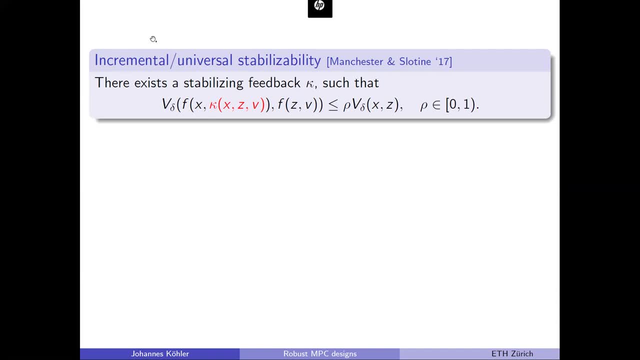 incremental universal stabilizability, and this essentially means that every reachable trajectory can be tracked by some controller, kappa. and since we also have disturbances, there's one last notion I have to introduce, and this is incremental input to state stability, which short delta is s, which can be characterized using corresponding control Lyapunov function. and now here we 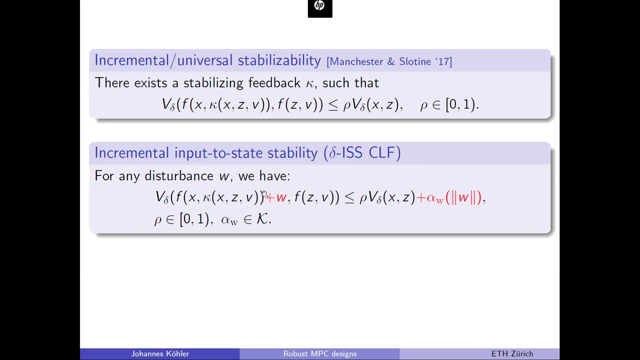 allow for an additional disturbance and we say the effect of this, additional disturbances- is bounded similar to a standard notion of input to state stability, only incrementally. So what does the system property mean? Roughly speaking, we have here a nominal trajectory. we have here another system which is subject to additive disturbances. 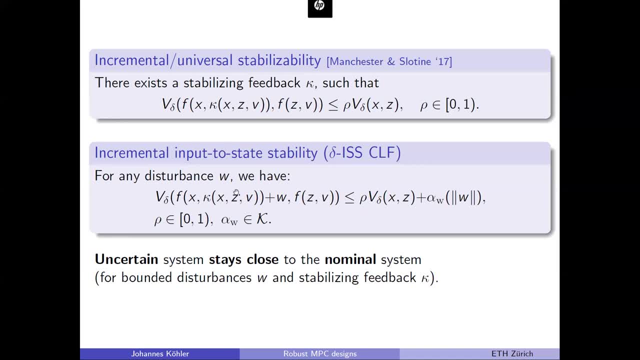 and we can somehow make sure with the system property that those two trajectories stay close even though we have disturbances, assuming that those disturbances here are bounded and we apply an additional stabilizing feedback. and this is kind of exactly the property. we need a robust prediction to be able to ensure that all uncertain predictions stay close. 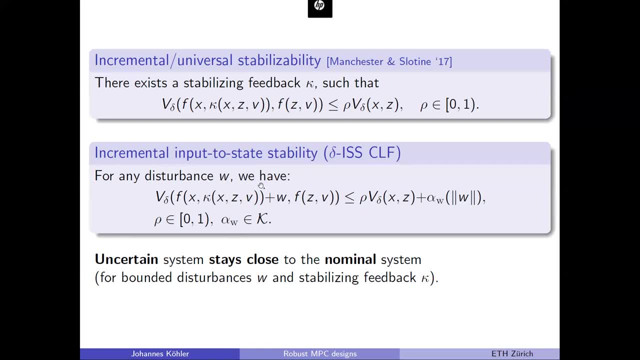 to some normal prediction, and this will also be the basis for the later framework and what I'll do next. I'll briefly explain how you can actually enforce or verify such a system property and compute a corresponding incremental Lyapunov function, and to do this we look at a 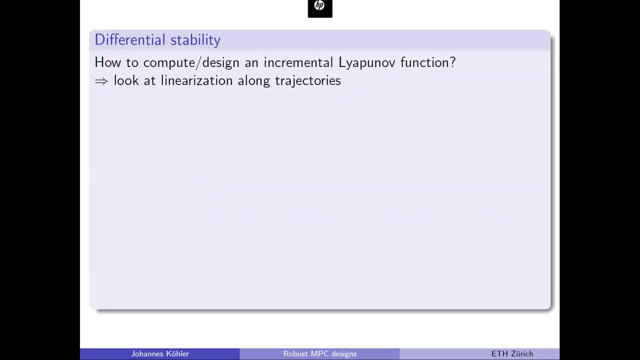 differential stability. so essentially, since it's difficult to directly work with nonlinear systems, we can linearize our system. now, since we look at stability of trajectories, now, we have to linearize our system along a trajectory. now, if we do this, what we essentially get is we have 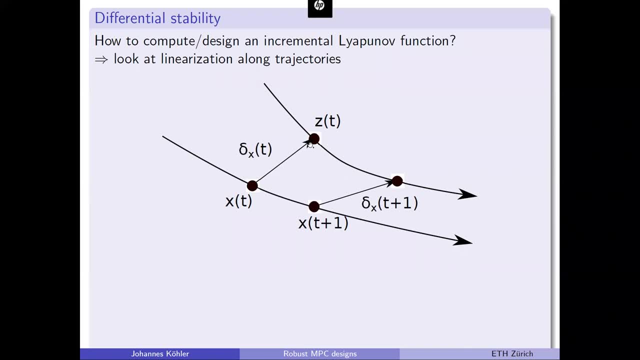 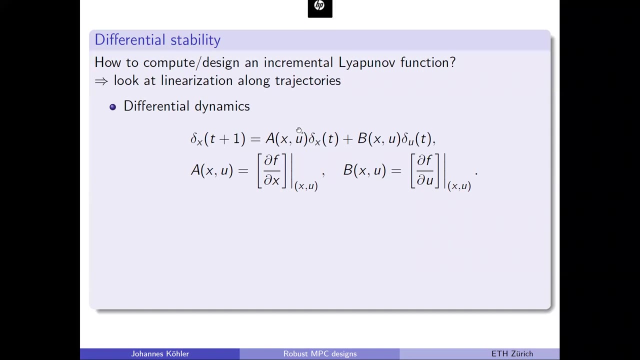 here two trajectories, and if we look at the difference between those two and make this arbitrary small, we end up with the so-called virtual displacement, and the dynamics of those virtual displacements are called the differential dynamics, and these are essentially linear dynamics where, however, the matrices a and b are given by the Jacobian, so they depend upon. 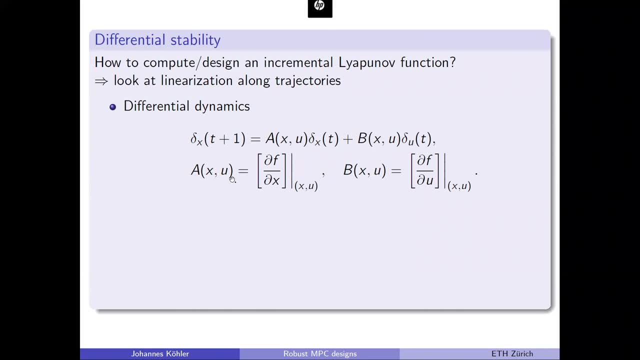 they depend on the state input around which I linearize my system. now we can analyze the stability of such a differential dynamic using differential Lyapunov functions, which are essentially quadratic Lyapunov functions of this arrow but which can also depend on the state, and those kind of differential Lyapunov functions are essentially equivalent to. 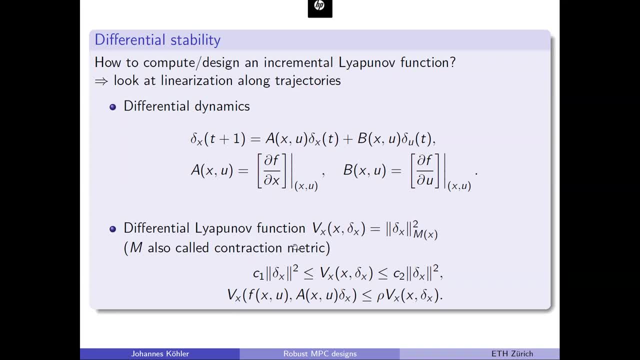 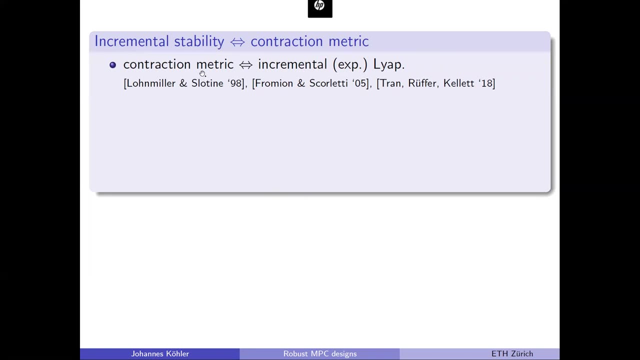 contraction matrices, and then stability is simply verified by having quadratic low and upper bounds and by having a contracting Lyapunov function. now why is this useful? the trick is now that we can use classical results from literature which say that if we can compute a contraction metric, 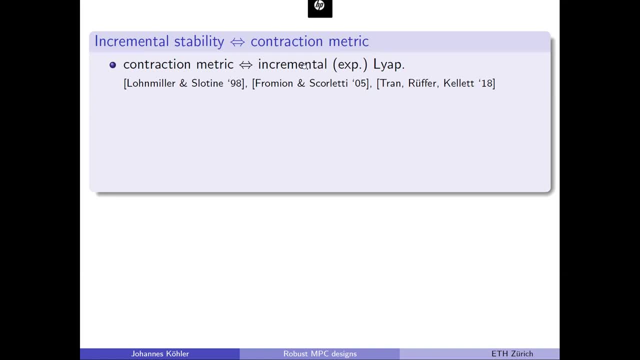 or a differential Lyapunov function, then we can also compute an incremental, exponentially stable Lyapunov function. there are some additional technical conditions, like continuous differentiability, but we'll not focus on them for now. so, in particular, if we have such a differential Lyapunov function or contraction metric, a valid incremental Lyapunov function is given by the. 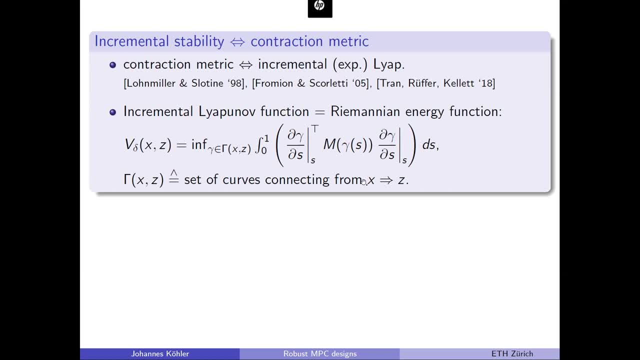 Riemannian energy function which is given by this function. here, and without going to details, we essentially look at all curves of the Lyapunov function and we can also compute a differential Lyapunov function with these curves that connect two points, and then we have here a kind of energy. 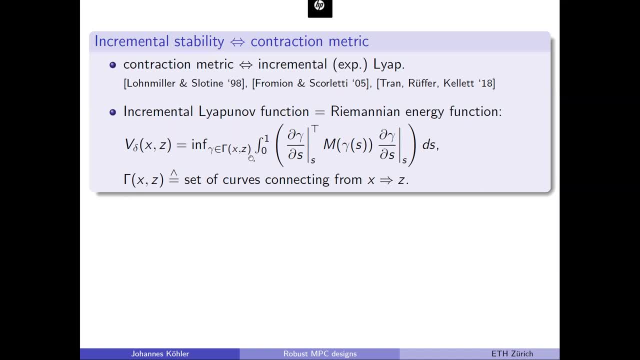 of those curves and we search for the curve of the smallest energy, which is also called a geodesic. and okay, without going into detail in the formula, one thing i'd like to note is that if this matrix here in the middle is simply a constant matrix, 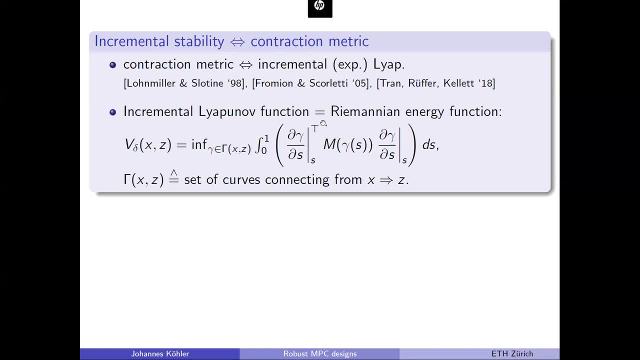 then this overall function would simply be a quadratic norm. so that's why for some special cases rate, but for others it can be very expensive. So what's important to note here is we can now compute incremental Lyapunov functions if we can find a contraction metric. The second important 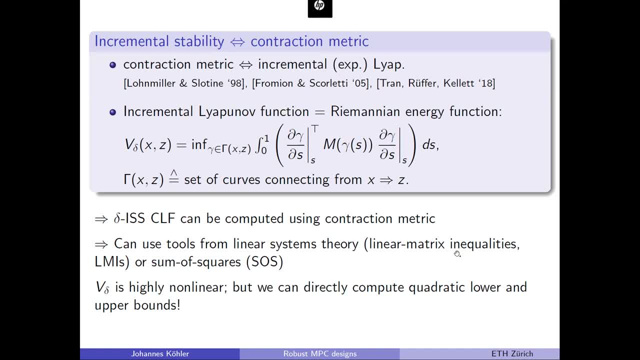 point is we can use tools from linear systems theory like linear matrix inequalities, but we can also use tools like sum of squares to actually compute such contraction matrices. But what's important to note is the resulting incremental Lyapunov function is highly nonlinear. so this is a very expensive to evaluate function But, what's also important, it's really easy to. 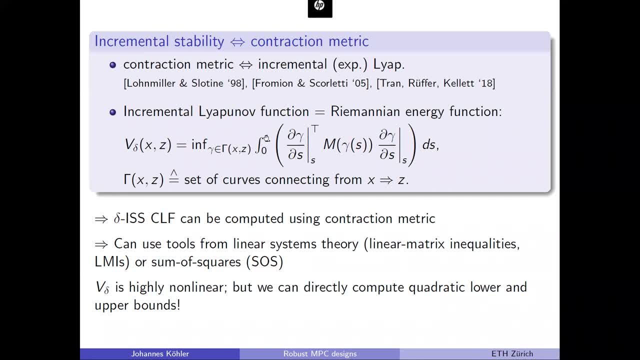 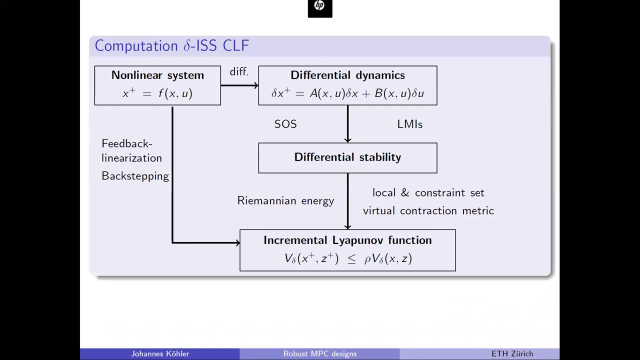 compute quadratic low and upper bounds on this function and that's why later we'll see, in the end we'll only need to use those bounds on the function instead of the function directly. Okay, so to summarize this briefly: we want to use incremental stability to do robust MPC. 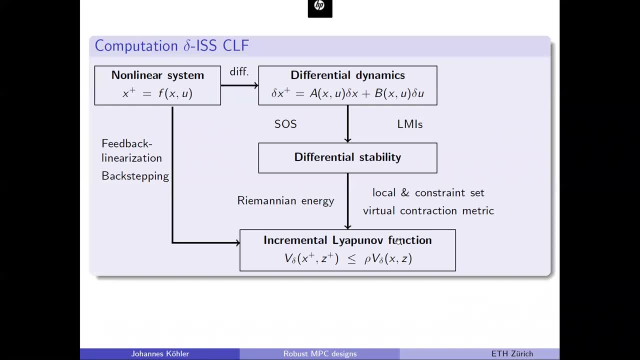 To get a corresponding incremental Lyapunov function. there are essentially two ways. The first way is to compute the function of the function. The second way is to compute the function of the function. Either we have a special system class like feedback, linearizable, or we can do backstepping. 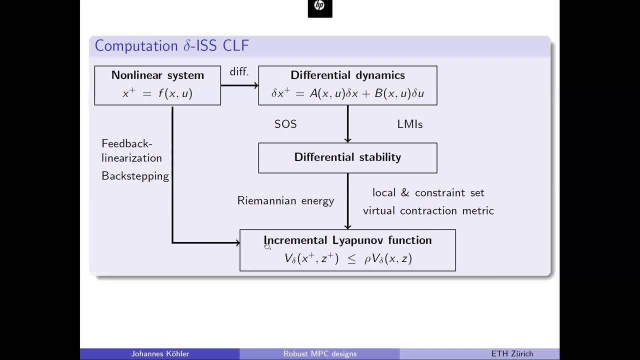 and then we can directly construct the corresponding incremental Lyapunov function. If this is not the case, then we can typically differentiate our systems and that with a differential dynamics. For this differential dynamics we can then find ensure differential stability using LMIs or sum of squares, and then with this differential 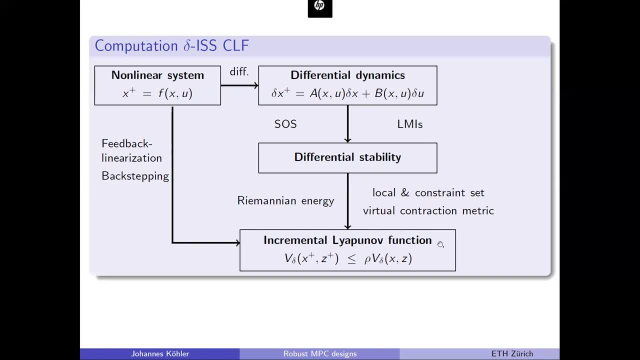 stability or contraction metric. we can compute the incremental Lyapunov function based on a linear energy, But also, especially if we consider constraints, there might, are some similar methods available, And with this we are essentially at a point where we can compute an incremental Lyapunov function. 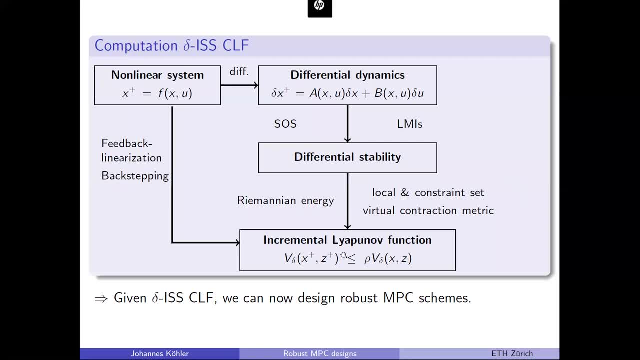 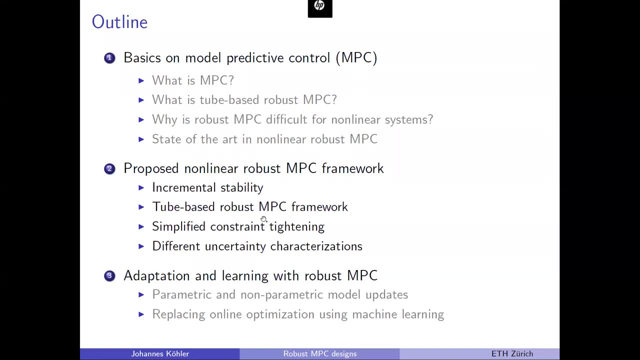 and now we will use the knowledge of this incremental Lyapunov function in the design of optimization-based controllers, And this will be the next step where we present a general cube-based, robust MPC framework. So the next step is to compute the incremental Lyapunov function based on a linear energy. 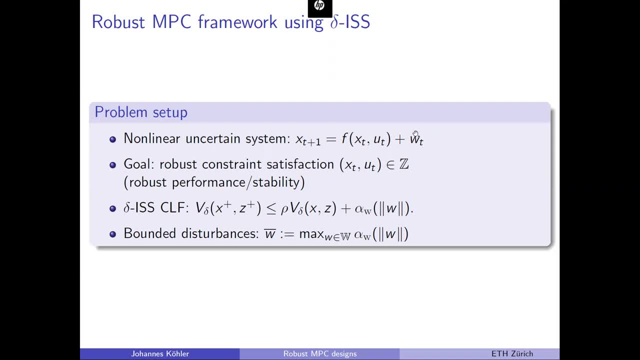 So the setup is as follows: We have a general non-linear system with some additive disturbances. Our goal is mainly now robust, constraint satisfaction of the state input, but similarly we can also ensure performance and stability. We assume that our system has such an incremental Lyapunov function. 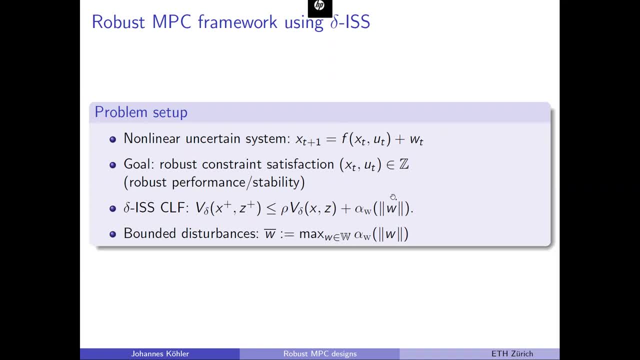 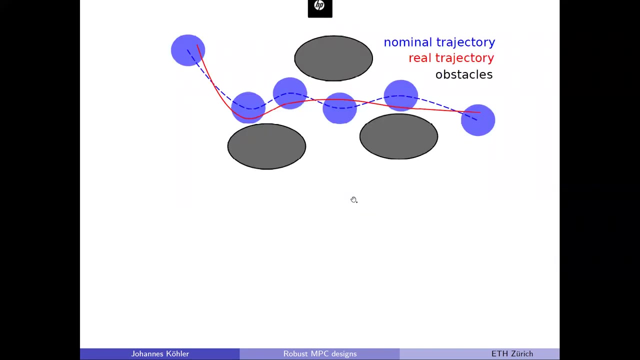 which is essentially exponentially contracting with an additive term depending on the magnitude of disturbances. And lastly, we assume that the disturbances are bounded, which means we can compute a scalar W bar over approximating this term here. Now recall: the idea in tube based MPC was that we construct such a tube of funnel around nominal. 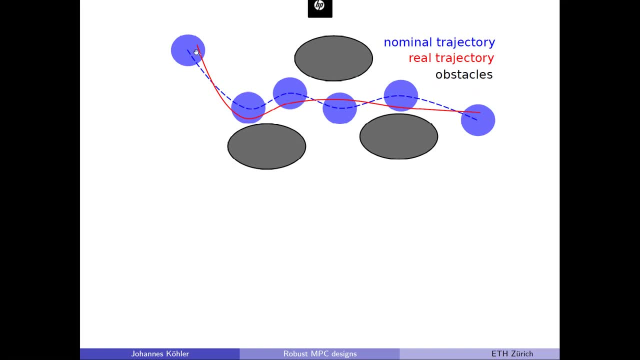 trajectories where the uncertain system will be contained in, such that we can do simple predictions with nominal models. And now the idea based on this incremental Lyapunov function is that these tubes or sets here are sub level sets of this incremental Lyapunov function, which are 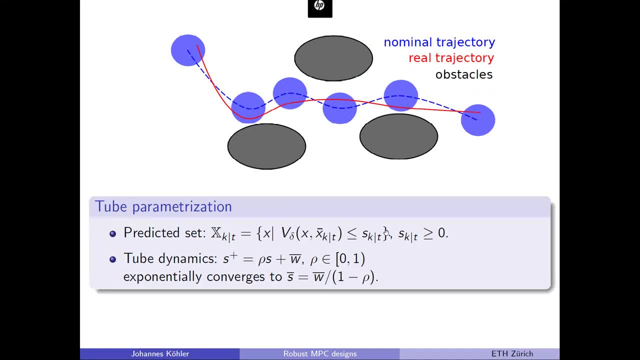 centered around a nominal trajectory here with a variable scaling. and the scaling which determines how large those cubes are is given by a simple scalar equation which is exponentially contracting, with an additive term, w bar, depending on the magnitude of the resistances. so what this means: as time goes to infinity, the size of this funnel or cube exponentially. 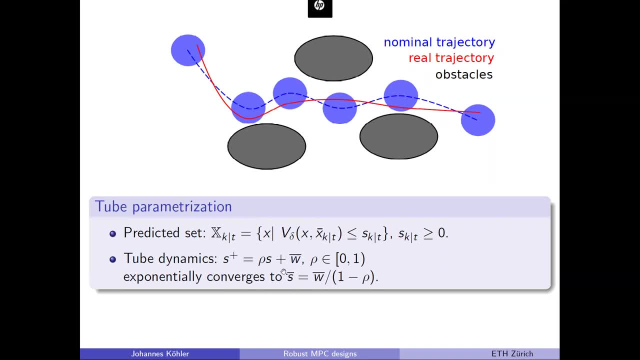 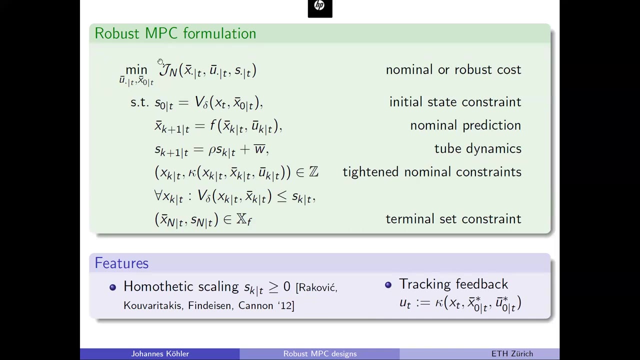 converges to some constant size. this means we can never have the case that the error gets arbitrarily large, but it will always remain bounded along a nominal trajectory. now, with this parameterization, we can formulate a corresponding predictive control formulation. in particular. what we do is now we, in addition to minimizing over 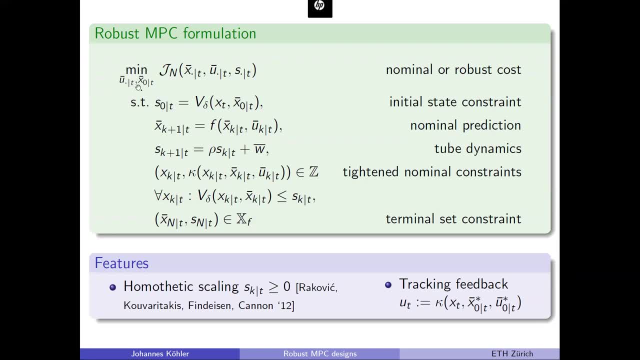 nominal input sequences. we also optimize over a nominal initial state. we minimize here some challenges: cost function. It could be just a nominal cost, but it could also be a worst-case cost. And now the first thing we do is we take the real measured state and this nominal state that 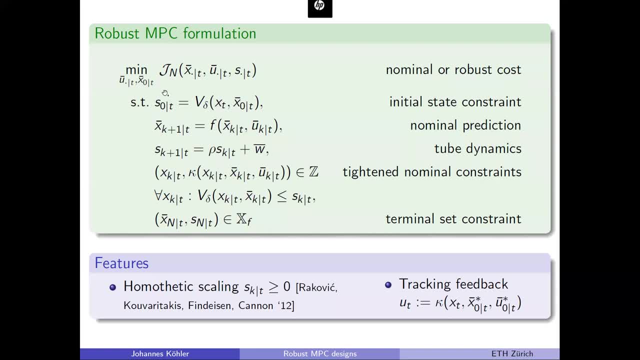 we optimize and we, based on this, we can determine the initial size of the tube where the real state is contained in. Then we can take nominal state predictions to predict our state in the future. We can predict the size of the tube based on the simple scalar. 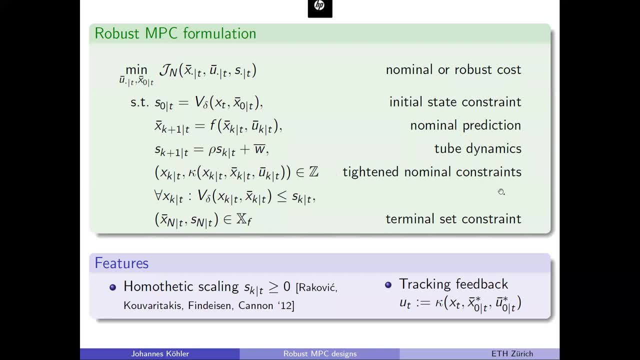 dynamics, And then here we have a set of tightened constraints which may look a little bit ugly, but basically what we ask is that for any state which is in this tube, the corresponding state and input should satisfy the constraints, And we'll see later how this can be efficiently reformulated. 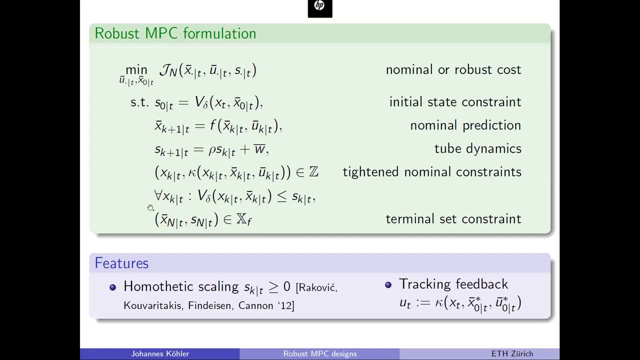 into standard constraints And, lastly, we might also have some terminal set constraint. Now, two things are important to note here. First, this is a so-called homophatic tube formulation, So meaning that those tubes we have around the normal trajectory are scaled with some scalar s, which is determined online, And a similar approach was also proposed. 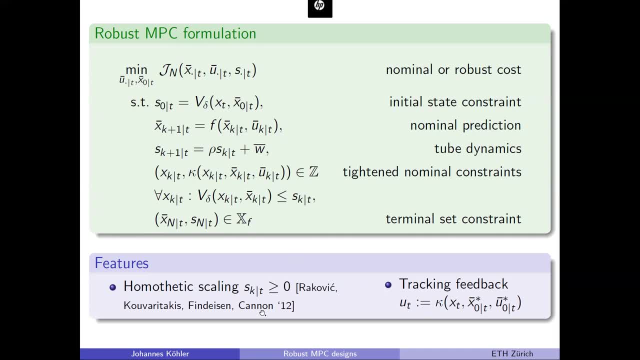 earlier in the literature for linear systems, And the main novelty is now that by using incremental Lyapunov functions we can also consider nonlinear systems. What's also important, since we compute here nominal trajectories which are not equivalent to the real measured state in closed loop, we actually don't apply the nominal. 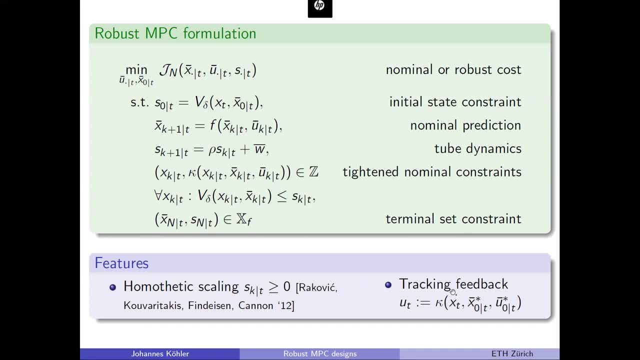 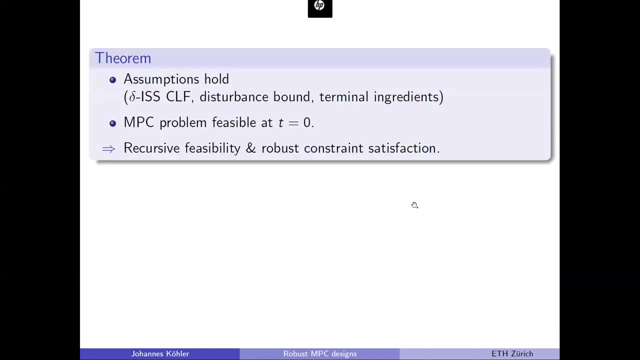 control input, but we apply a stabilizing feedback which drives our real measured state to the nominal trajectory. For this kind of a formulation we can directly derive our desired spherical guarantees. So if our assumptions hold, so that we have such an incremental Lyapunov. 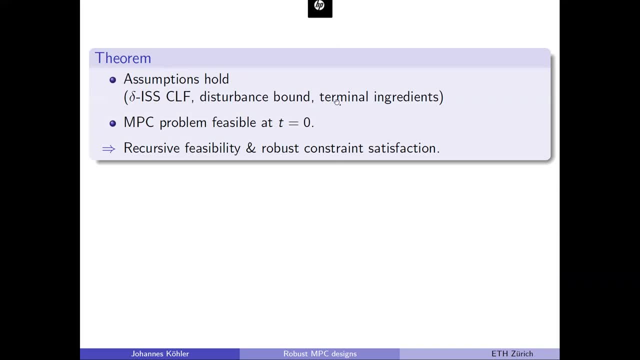 function, that our disturbance bound is correct and we have some suitable terminal ingredients- which I did not talk about too much- and we have that our optimization problem was feasible at initial time- then we can guarantee that this formulation will stay recursively feasible for all times and we will satisfy our constraints. I won't talk too much about the proof, but it's actually. 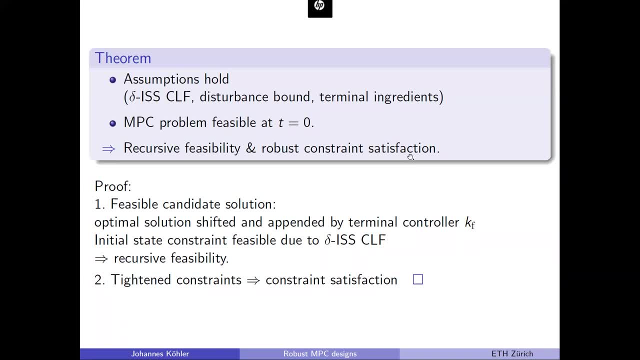 really simple because we have phenomenal trajectories. We can really choose a feasible candidate solution completely independent of the realized disturbance, and this will be feasible by our assumptions we made and the way we constructed this tube and the invariance conditions, And then by feasibility of this formulation and the way we define the titan constraints. 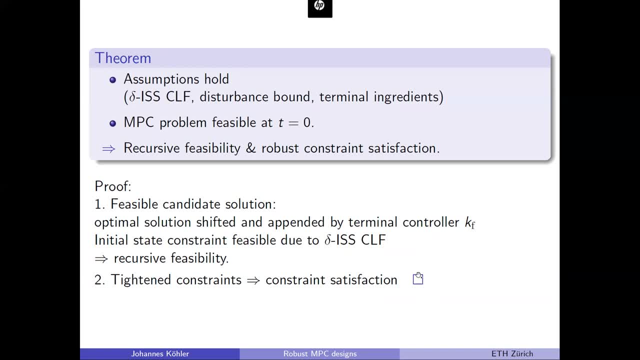 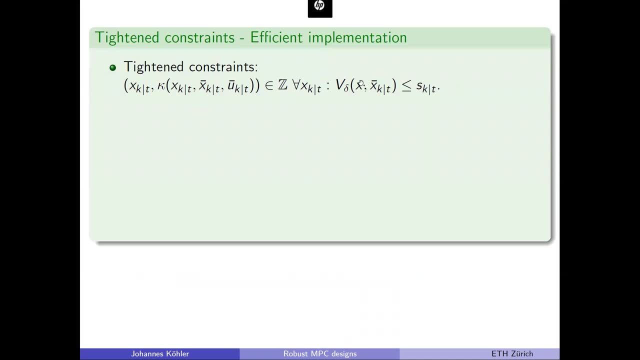 this also ensures that the real constraints are satisfied. Okay, now first, how can we actually implement this? So right now, I'm asking for every state which is in a sub-level set of a complex non-linear function- I wanted a corresponding state with the corresponding non-linear controller- should satisfy the constraints. And what we do- we typically 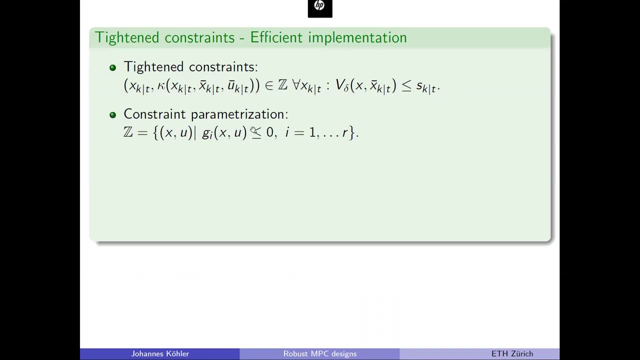 consider permutations where a constraint set is given as a set of inequality constraints And then if those functions here are continuous and this controller is continuous, then we can show a kind of continuity condition on this function that the difference between those constrained functions evaluated, the real state, and at the nominal state, is bounded by some function given. 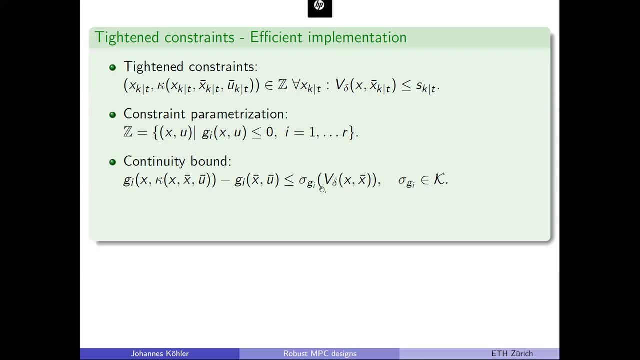 by the of the incremental Lyapunov function. So really the now uses continuity of your constraint sets. If you have hard collision, non-smooth collision avoidance constraints, it's also possible to deal with them. but you have to slightly desert work around, let's say. but you can still use those tube approaches. 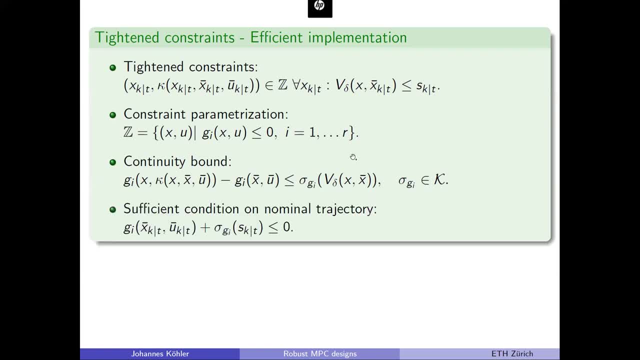 And now, with this continuity bound, actually your titan constraints are very simple. Instead of saying your constraints are g i's molecule zero, you know, say g i of a nominal trajectory plus a b of a nominal trajectory. So you can see that the constraints are very simple. 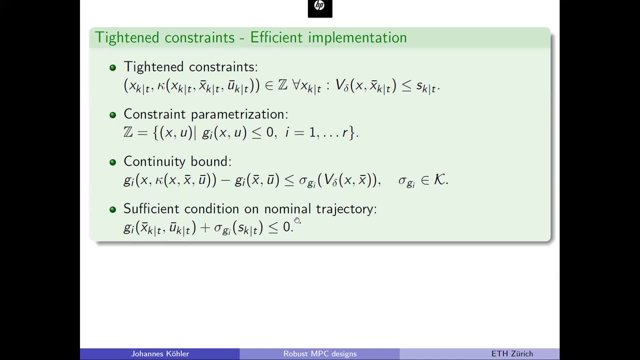 And that's the sufficient conditions and all the properties still remain. It was very important, so we just now implement the original constraints with an additional backoff. we computed online And this means the complexity of evaluating those titan constraints is essentially equivalent to the standard nominal constraints we had. 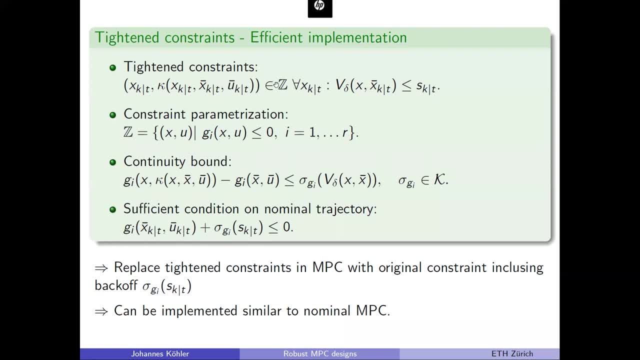 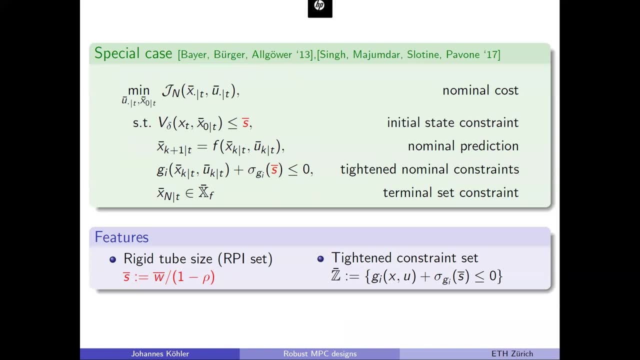 So really this titan constraints does not increase initial complexity. And what i'd like to note here, that's actually an important special case which was considered previously in the literature. That is, if we fix the size of our tube along the horizon to a constant size- so it's also called a rigid tube formulation- Then we can just remove those tube. 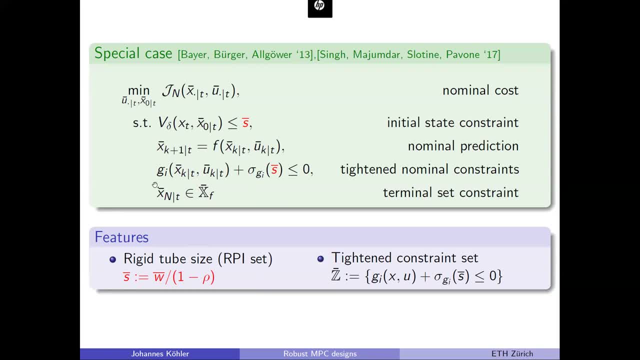 dynamics because it stays constant always, and then the formulation looks slightly shorter. What's important here? we can actually easily see that the titan constraints are very simple. We can see that the difference of this formulation compared to a normal MPC is only the first constraint where we have to have an additional constraint regarding it. 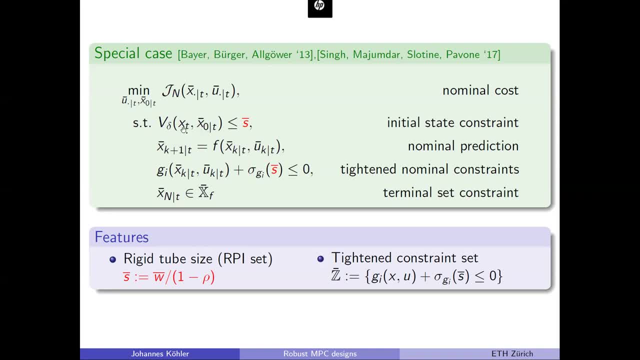 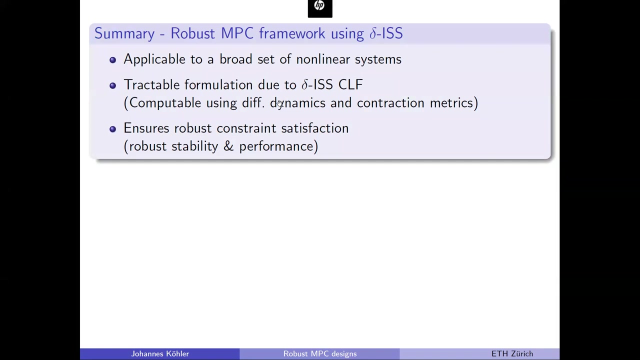 sorry, regarding a nominal initial state in a real measured state And here an additional constant which is added. So really the only thing that can add computational complexity here compared to a normal implementation is this first constraint here And this additional decision variable. Okay, so let me briefly summarize what i've done so far. 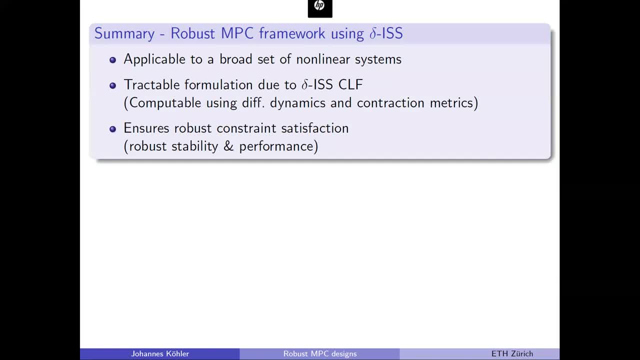 So we looked at a robust MPC framework using incremental stability. This is applicable to a rather broad set of on-l erste systems. By using such an incremental Lyapunov function we can get a rather subtractable formulation, And we also briefly discuss how we can compute such an. 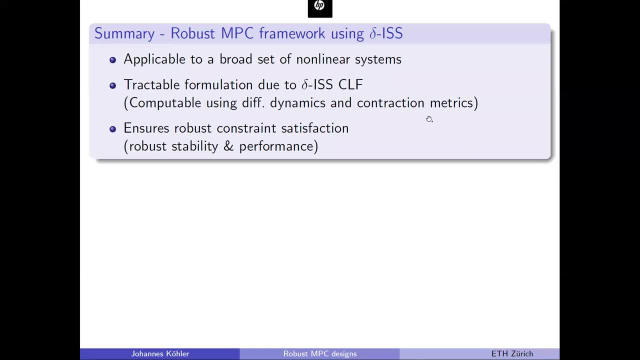 incremental Lyapunov function using differential dynamics and contraction matrices, And based on this, we could also ensure robust constraint. satisfaction, stability and performance can also be ensured similarly. Now, one problem with this formulation is actually this one initial state constraint I mentioned before, Because this initial state constraint involves the incremental Lyapunov. 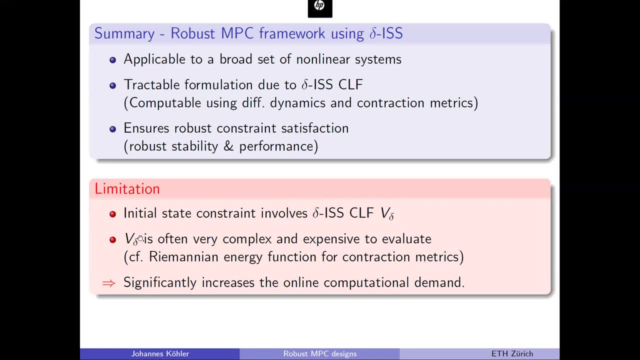 function And, as we saw previously, this incremental Lyapunov function can be very complex and non-linear, So evaluating this in the optimization problem can be expensive, And so just this one constraint might really increase our computational demand a lot, and it's of course not something we want. And to avoid this limitation we'll next look at a 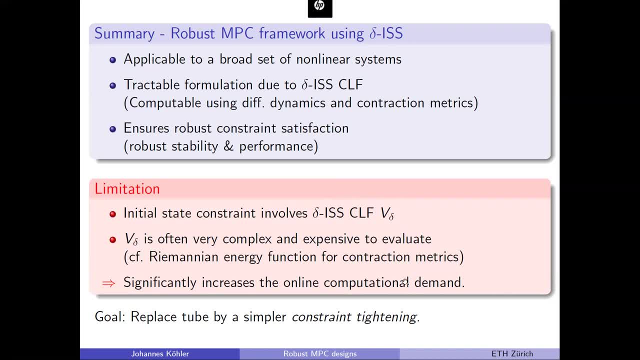 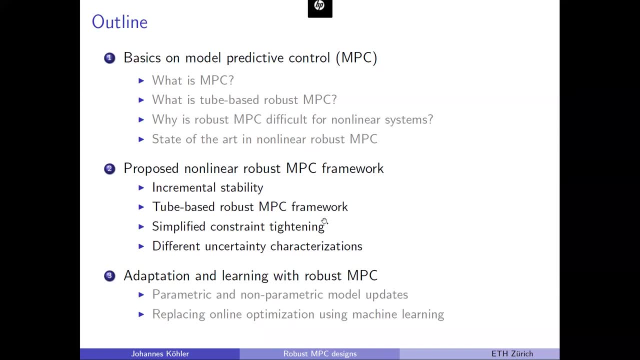 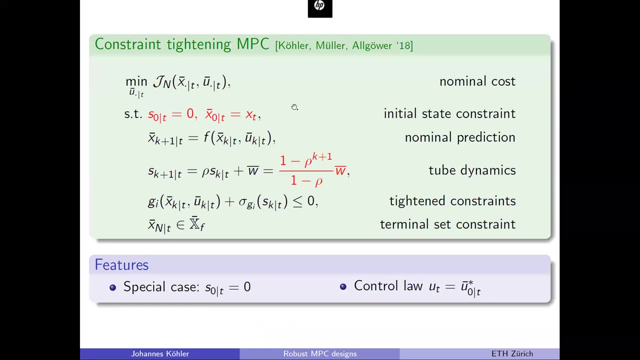 simpler constraint tightening. that just simplifies the formulation to get rid of this computational issue. And that's now this next talking point here: simplify, constraint tightening. The formulation looks as follows, And the main point here, what we changed compared to before, is that we now fix the size of our initial tube to zero, And this is equivalent to saying instead: 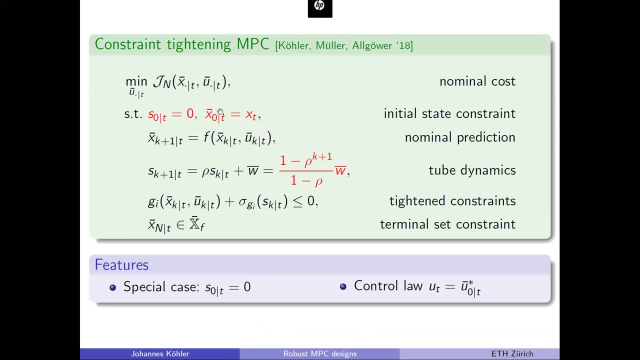 of having the initial nominal state as a free decision variable. we just fix it to be equivalent to the real measured state. And what's nice? by just taking this one additional restriction, the overall formulation now only has a nominal state prediction. The tube dynamics can be constructed offline. They're simply given by geometric series. 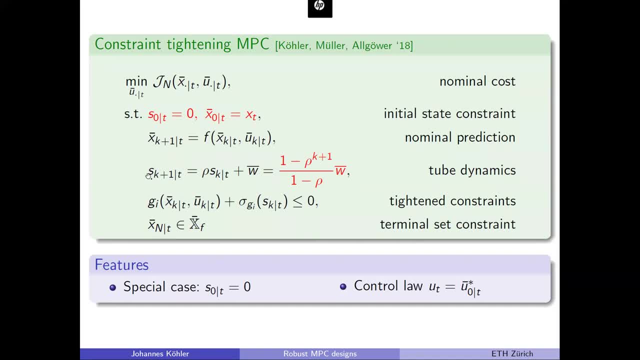 This does not involve any online computations. So the only difference to a nominal MPC implementation is now this one expression here, where we have a back-off in our constraints depending on the magnitude of the disturbances, which is varying along the prediction horizon. So that's really important And I think that's the main point I want to get across. 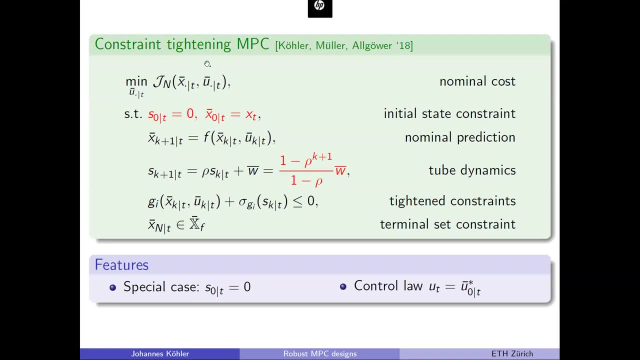 With this constraint tightening approach, now we only implement a nominal MPC with here an additional constant we computed offline, which modifies our constraints And, as we'll see in a second, this small modification will be enough to provide us all our guarantees, while it will not. 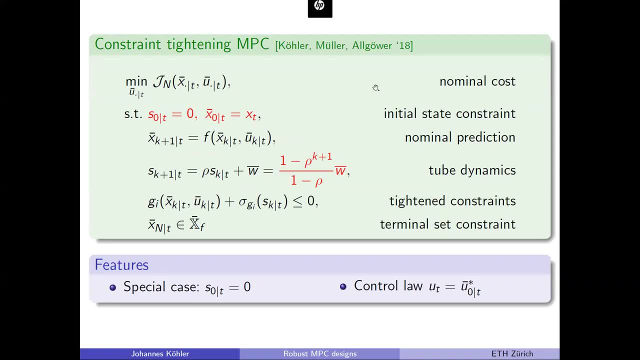 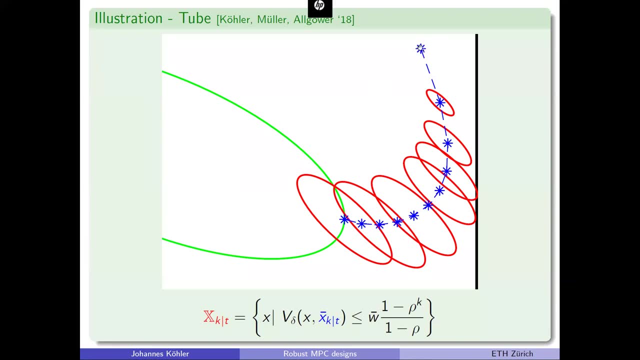 yield any additional computational complexity. As an illustration. so by fixing our initial state, the way the tube now looks is like this: We have here a nominal prediction in blue and now in the initial state we are actually 100% certain, certain where our state is. and then the future, those tubes grow larger, but also this growth is. 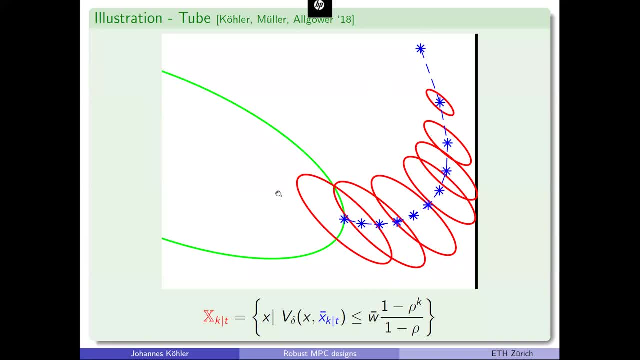 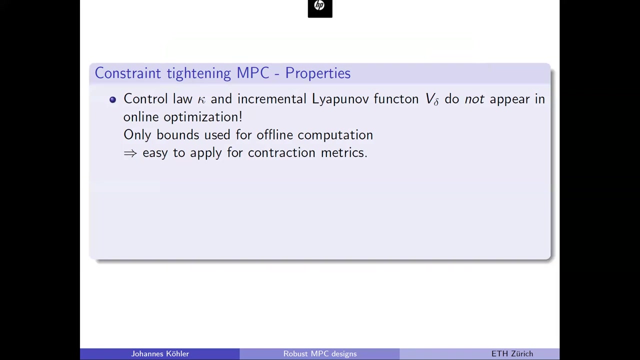 bounded and, yeah, then, does not grow to infinity. in particular, the expression for those tubes is simply given by this formula here, and we can see here, right, based on geometric series, how this will exponentially converge to some constant bound. okay, so what are the main properties of this approach? first, for the implementation of the 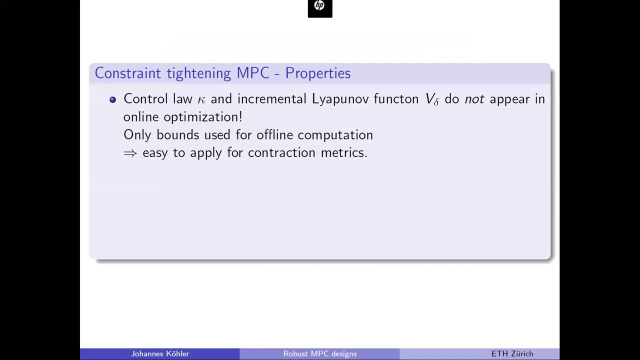 simpler constraint tightening. we don't use the controller assumed, nor do we actually use the function. instead, we only need to know that they exist and we need to know bounds on them. we never need to evaluate them, and this is particularly useful if we work with contraction matrices, where the inclusion of the McDonald's contractions is 현재 and we are using the. 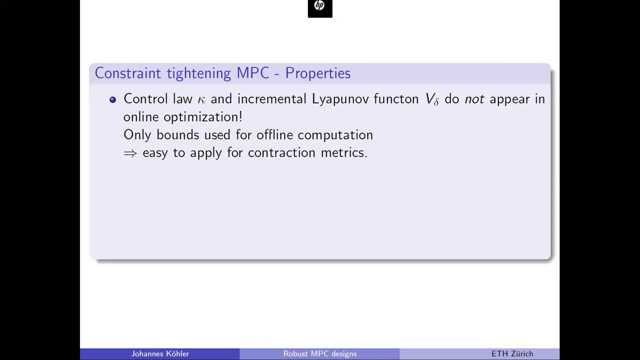 increase in the acceleration coefficient, which is the think um function and the objective to just incremental Lyapunov function is expensive to evaluate but we can easily compute bounds on the incremental Lyapunov function. But I also want to stress again the resulting computational complexity. 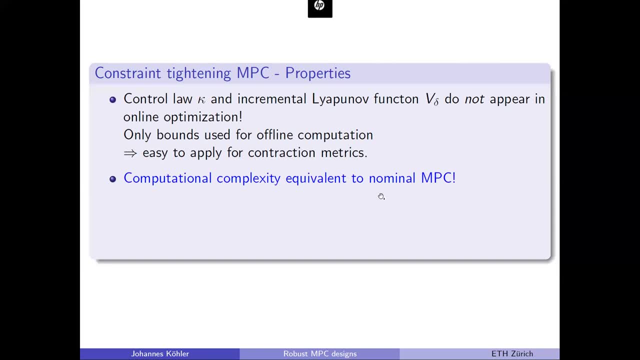 of this constraint-tightening MPC is now equivalent to a nominal MPC, meaning the same number of constraint function, variations in the constraints and cost function. And also, as a special case, we directly get the Lipschitz-based constraint tightening which was proposed previously in the literature. 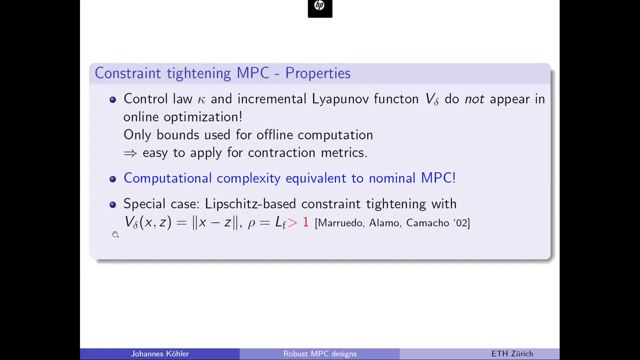 And this would be a simple case where we just replaced the incremental Lyapunov function by a norm and we would replace our contraction rate, rho, with a Lipschitz constant. And here we can see why, of course, if we work with contraction rates, 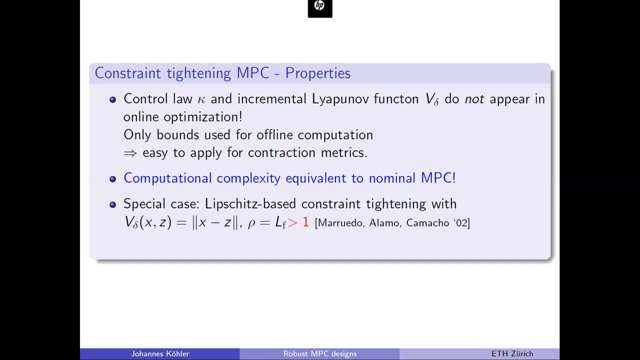 we have a constant smaller than one, which gives us some boundedness on the error, while if we work with Lipschitz constants, which will typically be larger than one in a discrete time case, you can only get unbounded bounds on the error. 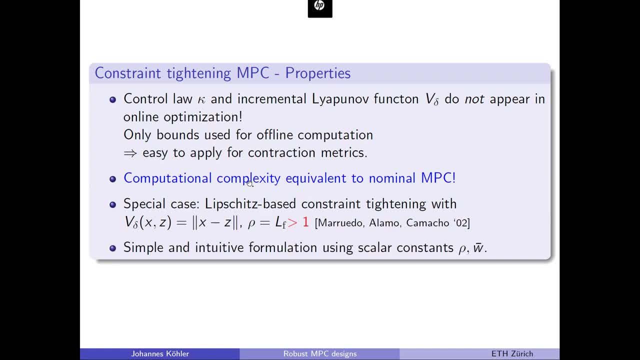 which will be very conservative for large horizons. And the last point I want to mention, actually for the overall formulation, there are kind of mainly two tuning variables which makes it really easy to implement. One is a system constant rho, which tells us how fast we can stabilize our system. 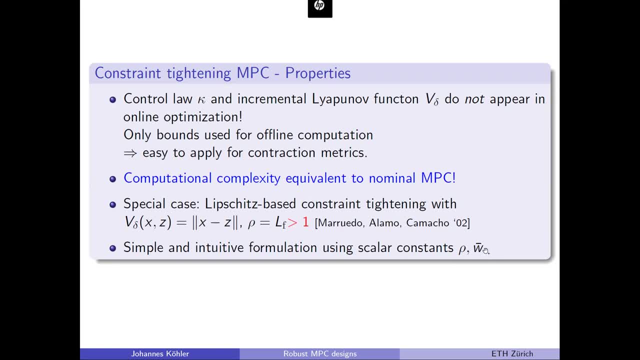 And the other is a scalar W bar which gives us a bound on the magnitude of the disturbances, And this, of course, makes it very easy to online tune if we are uncertain about the exact magnitude of the disturbances. For this formulation, we also have a corresponding vertical result. 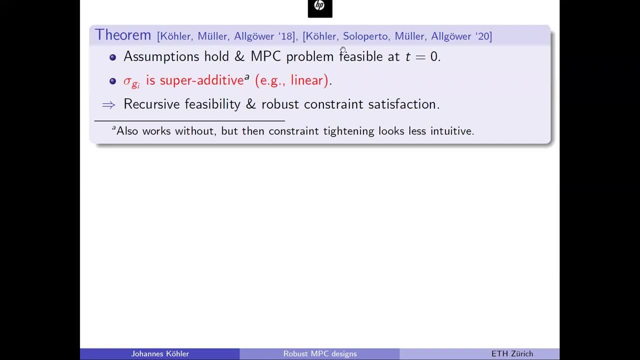 So if we have the same assumptions as before and the FTC is feasible at the initial time, we have a small additional condition, which is here that those functions describing the continuity of the constraints are super additive. So, for example, if we have Lipschitz continuous functions, 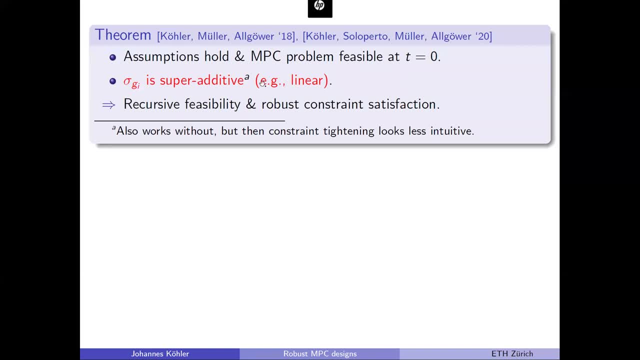 then this holds a linear function. Yeah, but this is actually only an assumption to simplify the exposition here. So you can also work with all this assumption. then just the MPC formulation looks slightly different, but it's not the real restriction. And now, with those conditions, 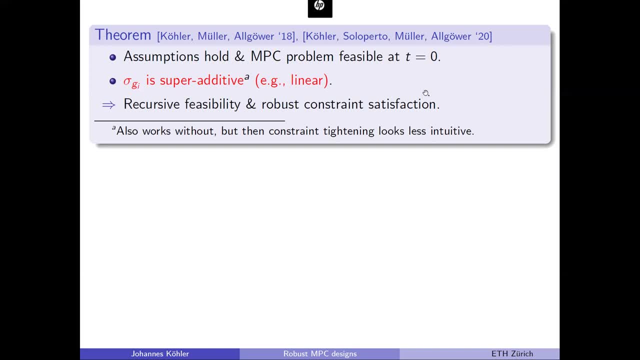 what we get is we can ensure recursive feasibility and robust constraint satisfaction. And, very briefly, there's one thing I want to note about, a proof, and this is what the actual candidate solution is that we use, In particular because the measure state is now equivalent to the 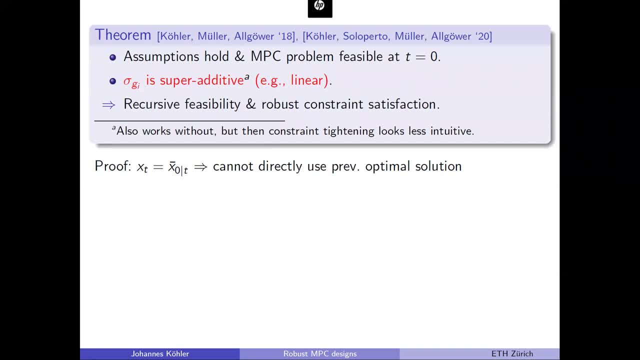 our nominal state is equivalent to the measure state. we cannot use the previously optimal solution as a candidate solution, which is what we usually do in most MPC proofs. So instead, what we do is we say, as a feasible candidate solution, we want to track our previously optimal solutions. 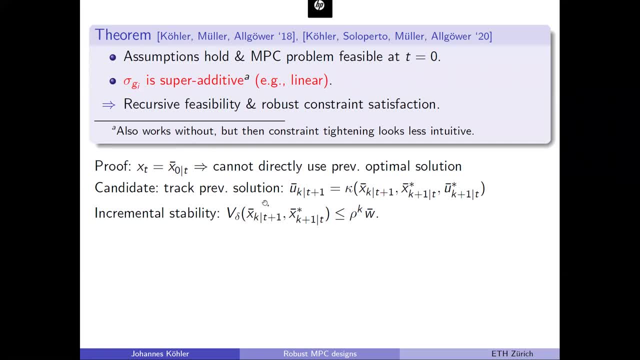 And because our system is stabilizable by assumption, we know that somehow the distance between this new candidate and the previously optimal solution is bounded And based on this we can easily work out that again, we can easily work out that actually all the constraints 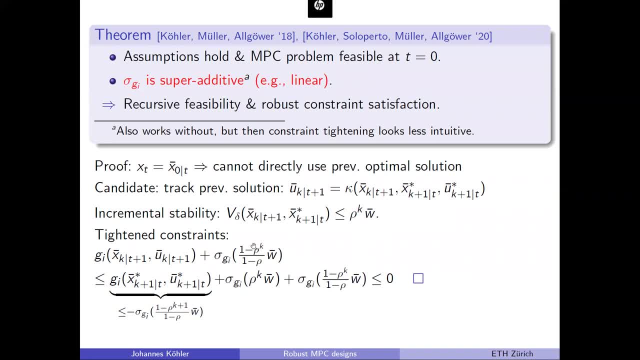 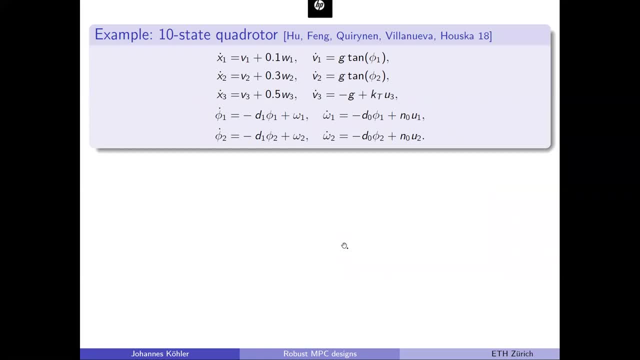 are recursively feasible, And this is essentially only a geometric series arguments. Okay, let me briefly show an example that's actually applicable. So this is a 10-state crash helicopter taken from literature. It's not too non-linear, It's mainly taken because it has a medium-large state space. 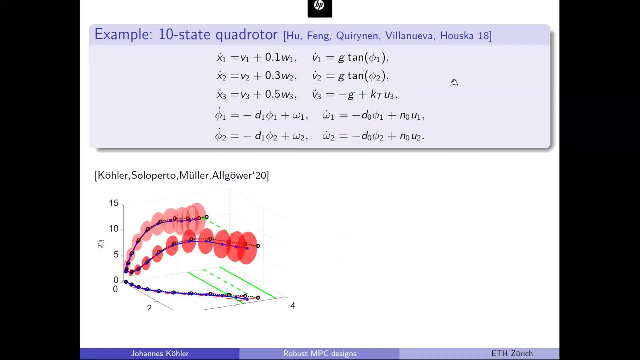 to show that it actually works for not only small-scale systems. And here we can see an example of a cross-spanning closed-loop plot. So we have here, blue, a nominal trajectory and here in red, those ellipses around it are the tube which contain all uncertain trajectories. 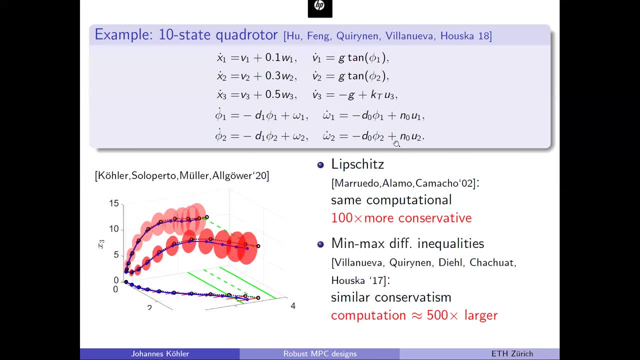 For this system. there are also other methods that would be applicable, So one could also use Lipschitz-based constraint tightening In both cases. the proposed method and the Lipschitz-based constraint tightening have the same computational demand as a nominal MTC. 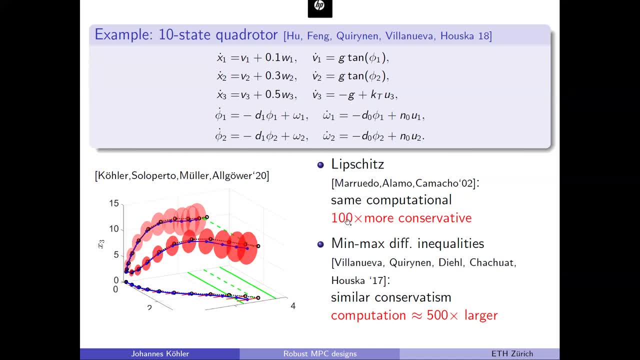 But the difference is here: the Lipschitz-based constraint tightening is 100 times more than the normal MTC. It's more conservative And the reason for that is that the Lipschitz constant to the power of the prediction horizon is a very, very large number here. 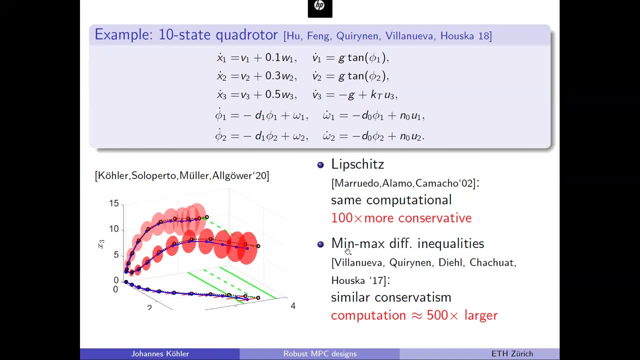 which makes it very conservative. One can also consider here min-max differential inequalities. This is where those ellipsoidal tubes are computed online. For such an approach, we can achieve a similar conservatism. but the main difference is that, since this approach optimizes ellipsoidal sets online, the number of ellipses. 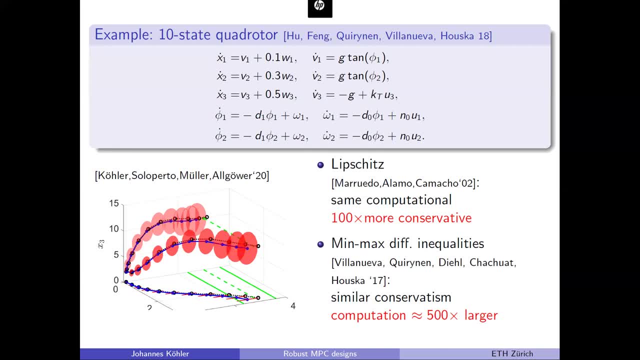 the number of decision variables are 10 by 10 matrices over the horizon, And because of this the computational demand becomes 500 times larger compared to our approach. So really we can see, at least to those two formulations we compare rather favorably. 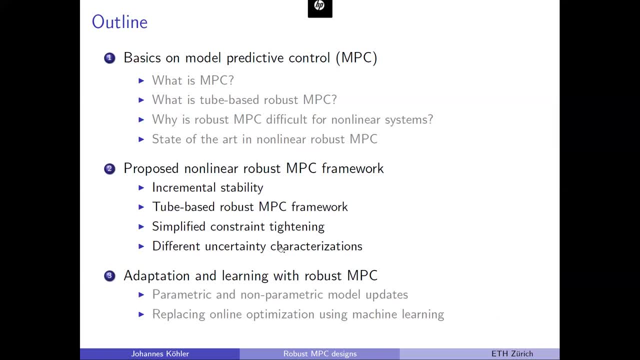 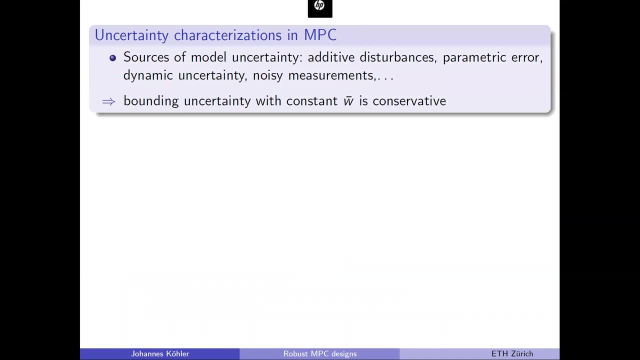 OK, this brings me to the last point I want to mention regarding robust MTC, And this is different uncertainty characterizations. So in all practical applications, we essentially, you know, we essentially have various sources of model uncertainty. We can have additive distances, parametric errors, 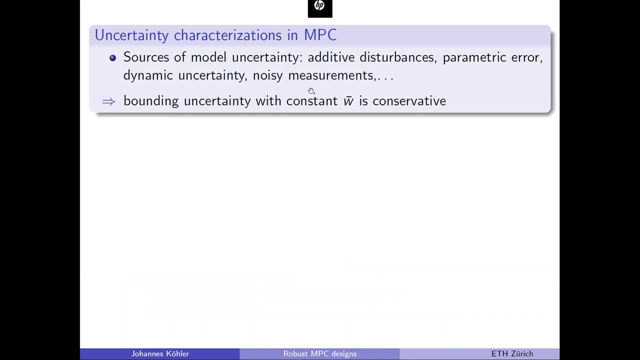 dynamic uncertainties, noisy measurements and a lot more. And now, if we bound all of this uncertainty with a constant scalar, this can be rather conservative. So this is what we've done before. It is also what most robust predictive methods do, but this can be conservative. 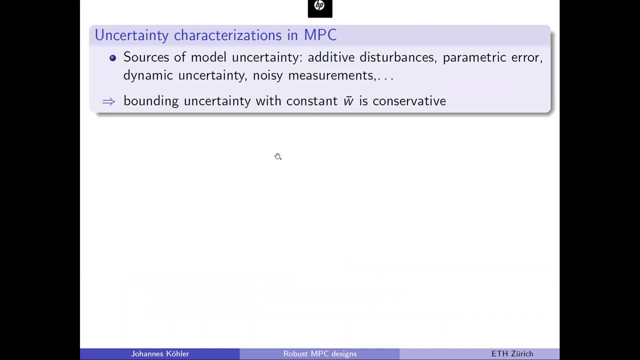 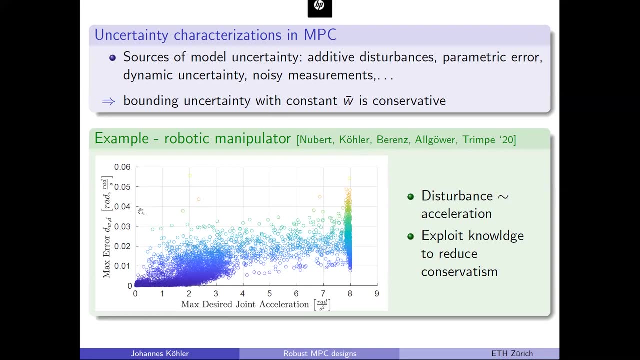 And our question is: how can we do better? And just to give an example of why this is relevant, this is also taken from the you know robotic manipulator I showed you at the beginning. We have experimental data regarding mesh model mismatch. 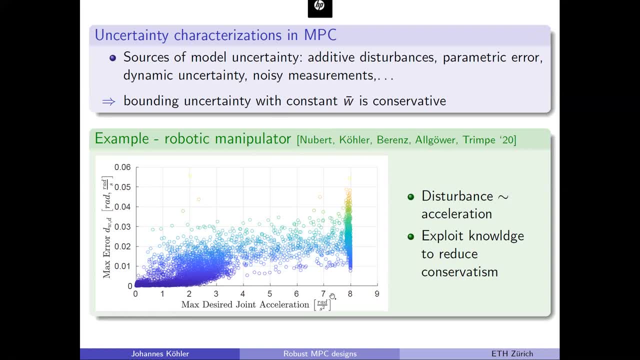 and here an acceleration And what we can see. first, if we have no acceleration, that's essentially no model mismatch. And if we increase the acceleration, then our model mismatch for increase And I would say this is not too surprising and this is also something which we 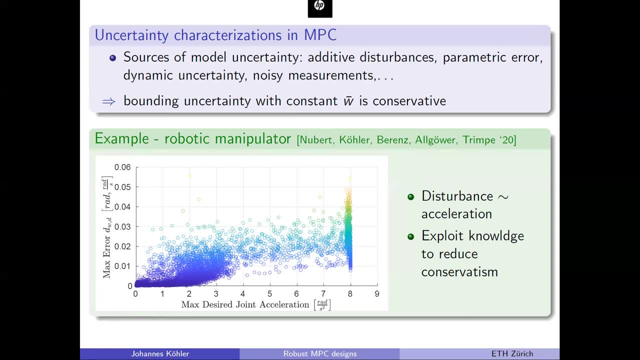 can see in a lot of applications, And if we now use a constant bound on uncertainty to characterize this, then we Sud pants change. Then we have to use a very high bound to get robust guarantees Or we would have to limit our acceleration to small values to get a smaller bound. 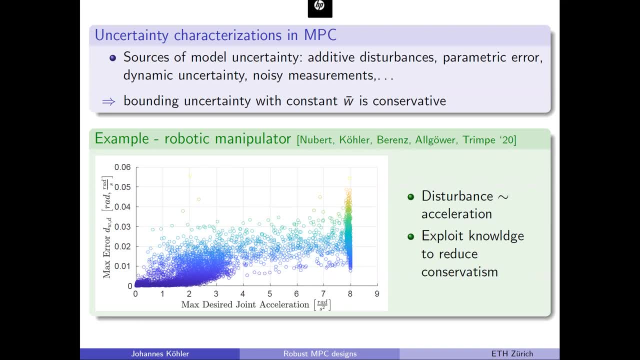 And both of those are, of course, not ideal, And what I want to talk about next is how we can directly use a bound that, for example, uses the shape of how high the disturbances can be, which depends on how high the acceleration, for example, is. 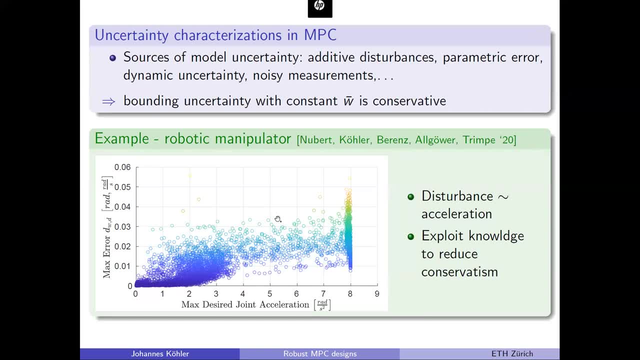 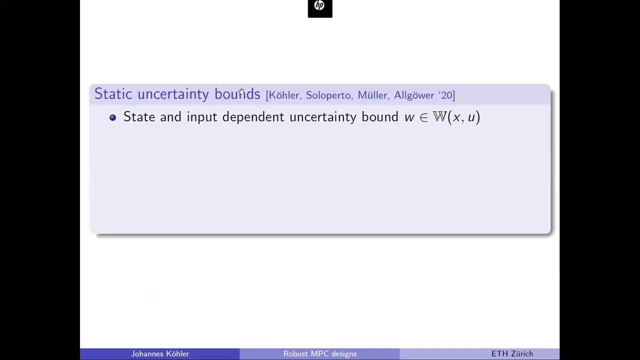 And by using this we can use more knowledge and thus reduce conservatism. The main thing I want to focus here on are static uncertainty bounds, So everything which is not dynamic, And this essentially means all bounds which only depend on the current state and input. 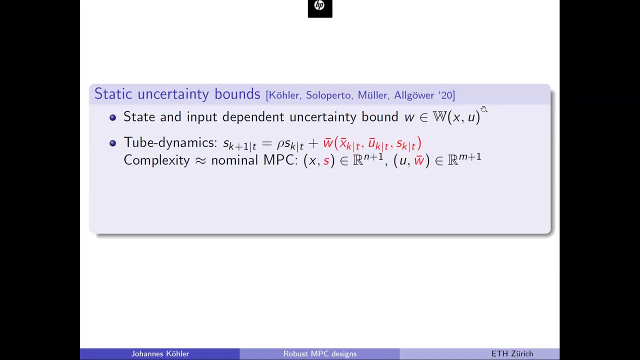 Now, if we have such a bound, then we can simply replace the previous formulation. We still get the same tube dynamics. So the next time step is contrasting. And now, instead of having an additional scalar bounding the uncertainty, we have here a nonlinear function, W bar, which depends on our nominal trajectory and the tube size. 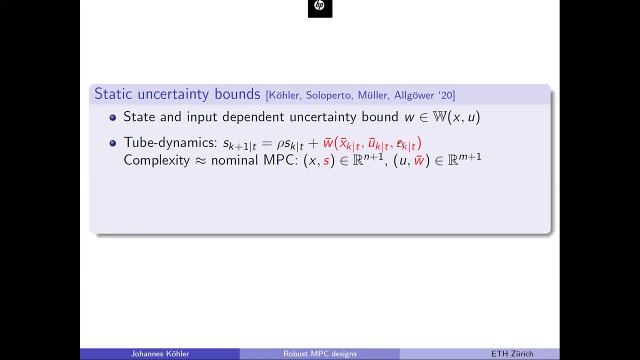 And now this nonlinear function here needs to be chosen in such a way that it over-approximates all possible model mismatches for all states and inputs in the tube, And we'll see in a second how this can be practically implemented. But what's now important with this additional tube dynamics? 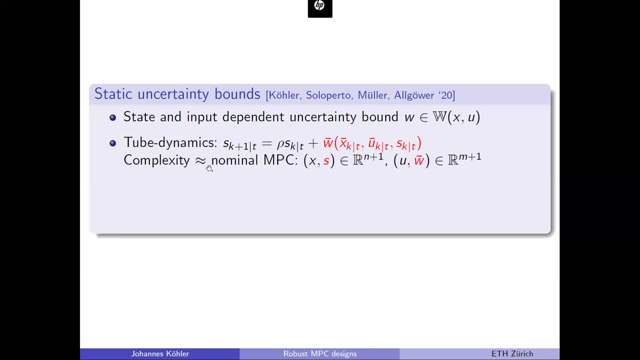 In those general static uncertainty bounds, the resulting computational complexity can be written equivalent to a nominal MTC which has one additional scalar state, particularly here this tube size, And we can implement with one additional scalar control input which is used to evaluate this nonlinear function here. 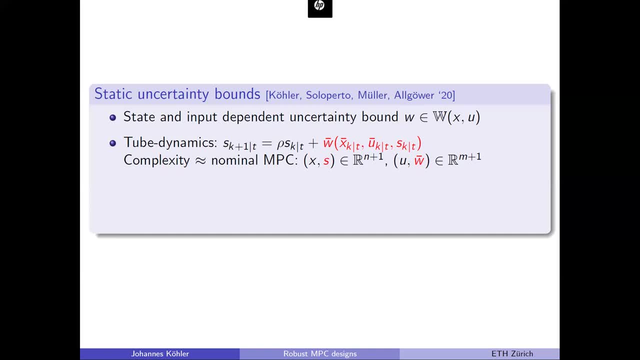 And so with this, actually the online computational demand increases, but only moderately and particularly only with one scalar state input dependent. And to give you an example, the most standard case would be if we have a quadratic Lyapunov function and our model mismatch is parametric error, so it's something linear in parameters and, for example, this parameter is contained in a polytope. 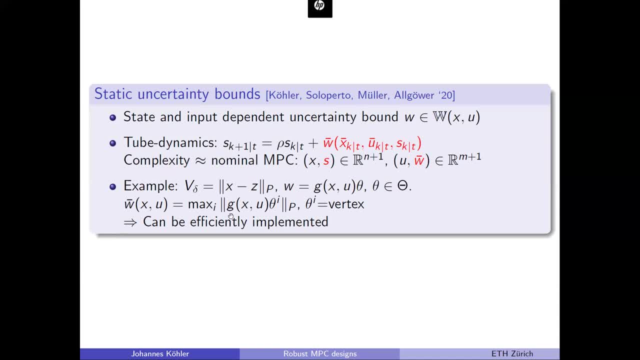 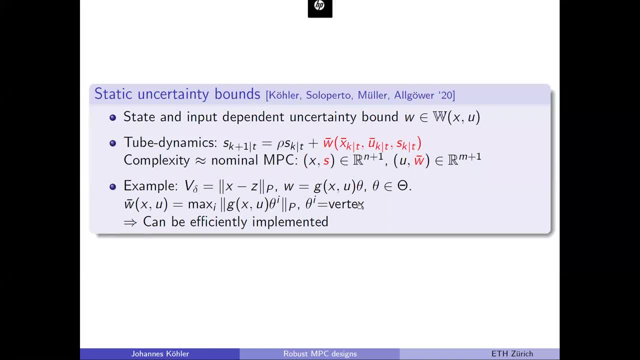 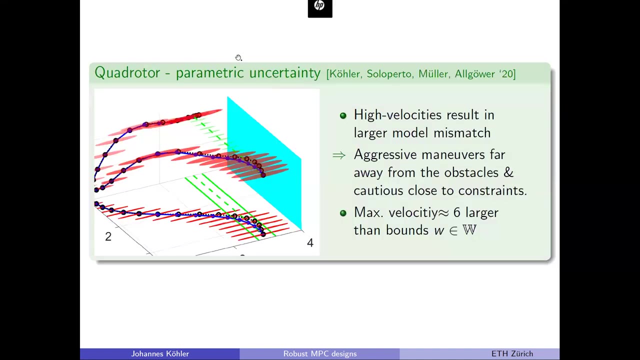 Overall parameters, which can be implemented by enumerating all vertices, and this can be implemented as multiple inequality constraints in the MTC. So overall, we can still use standard implementation methods to deal with this. And here's now an example. It's again the same protocopter from before, but now we have some parametric mismatch. 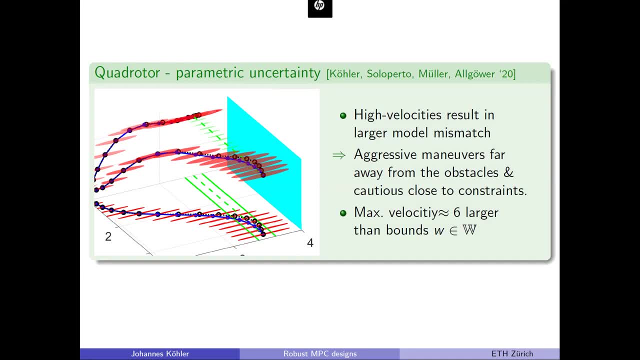 And because of this parametric uncertainty, we get that if we drive with high velocities we'll get a larger model mismatch, Which is something which is the case for a lot of practical applications. And now MTC knows this and uses this knowledge in the predictions and as a result, we get that we allow for aggressive maneuvers if we're far away here from our obstacles, but we'll automatically be more cautious if we're closer, because then we have to reduce the size of our tube. and uncertainty. 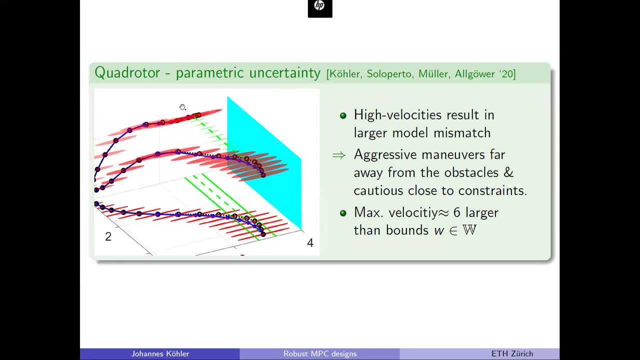 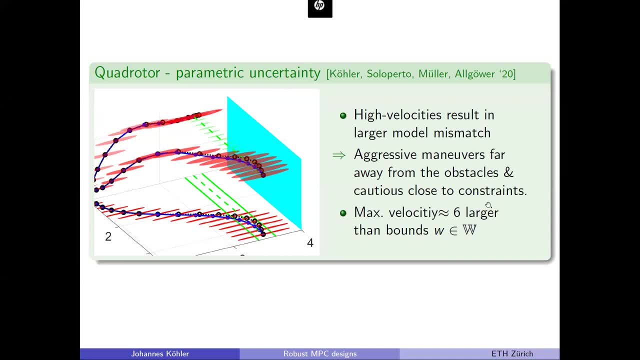 And in this particular example, if we would instead use a constant bound to describe the model mismatch, we would have to reduce the maximum velocity by a factor of six. So this shows really that there's a huge potential by using non-constant disturbance characterizations. 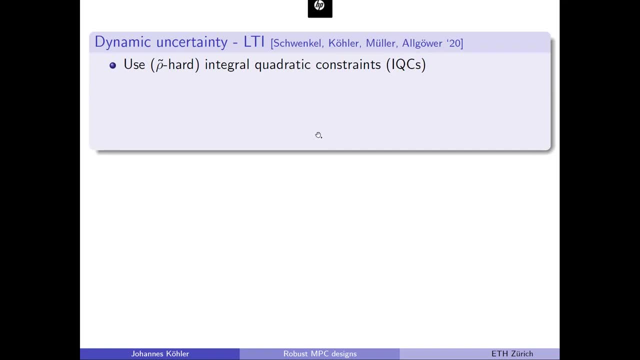 Very briefly, I want to mention two other classes of uncertainty. we can consider One. the most general would be dynamic uncertainties. This is a rather recent work and so far only for LTI systems, But essentially what you can do is you can characterize dynamic uncertainty. 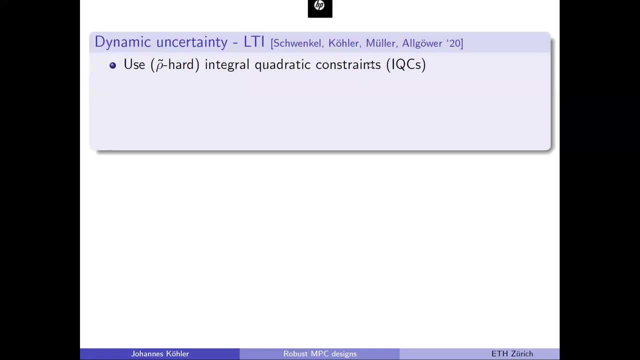 But essentially what you can do is you can characterize dynamic uncertainty, like delays, using integral quadratic constraints, which is one of the standard tools from robust control theory. Then, instead of using an incremental Lyapunov function, we can characterize the tube with a control Lyapunov function from the IQC theory. 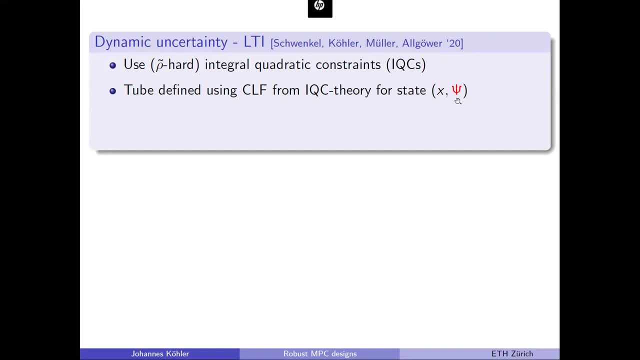 An augmented state given by the real state and some filter states which characterize those IQCs And then the actual implementation. we again get similar tube dynamics And then the actual implementation. we again get similar tube dynamics with some scalar here, some contraction rate- rho, tilde now- which comes from those IQCs. 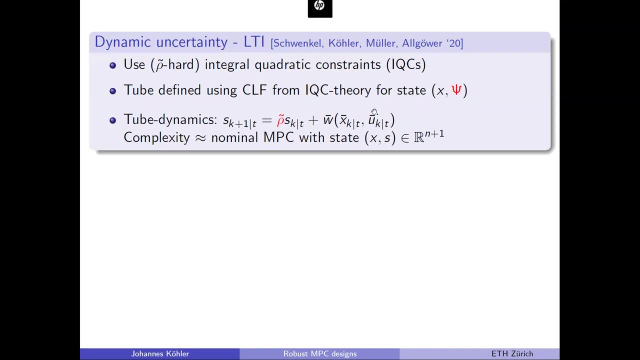 and again on some nonlinear function depending on our nominal trajectory. And so overall you can again implement this similar to a nominal MPC scheme with an additional scalar state, so only moderately increasing the computational complexity but dealing with dynamic uncertainties. And similarly we can also deal with noisy output measurements by doing a set-based estimator. 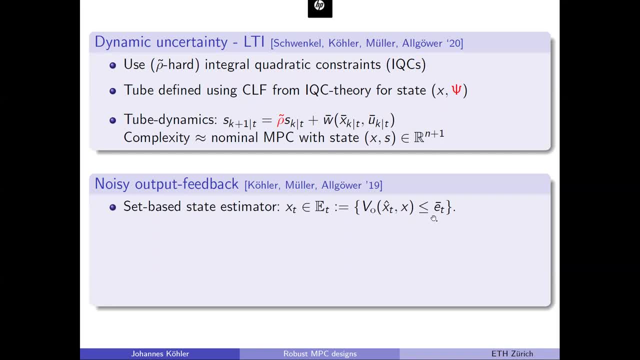 which contains the error for all times, So this is easy to compute, for example for Lundberg Observer. Then we use some predictions on how high the estimation error will be in the future, And then we can find some simple formulas that can be implemented. 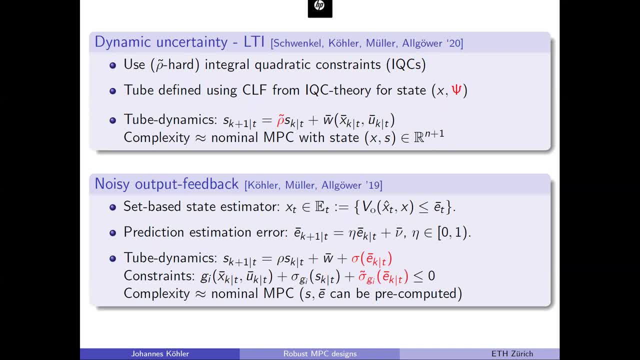 And we essentially get exactly the same computational demand again as a normal MPC, But we can incorporate additive distances, noisy output measurements and estimation error. Okay, This brings me to the last part. Okay, This brings me to the last part. This brings me to the last part. 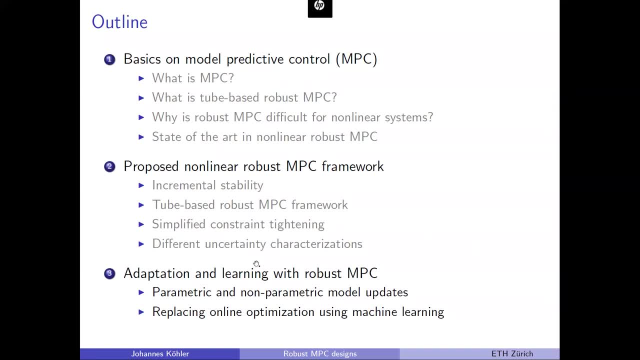 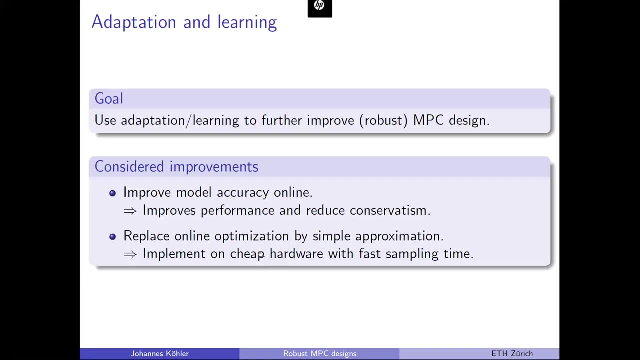 This brings me to the last point of this presentation, where I briefly want to talk about how adaptation learning can be used to further enhance robust MPC formulations, And for this, there are two different things I want to look at. One is improving model accuracy online, and this will help us improve performance and reduce conservatism. 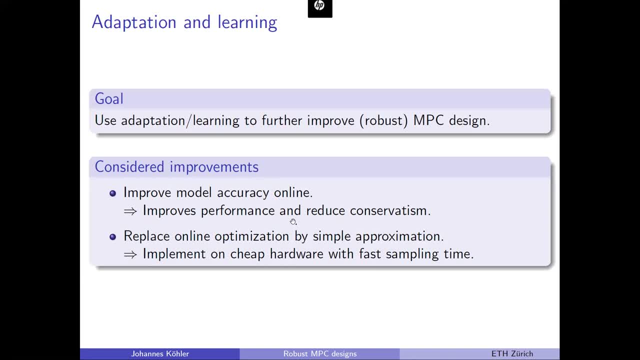 And the other thing will be to replace the online optimization with simple functional approximations, And this will make it a lot easier to implement MPC schemes on even cheaper hardware, while injuring faster sampling terms, And this will make it a lot easier to implement MPC schemes on even cheaper hardware. 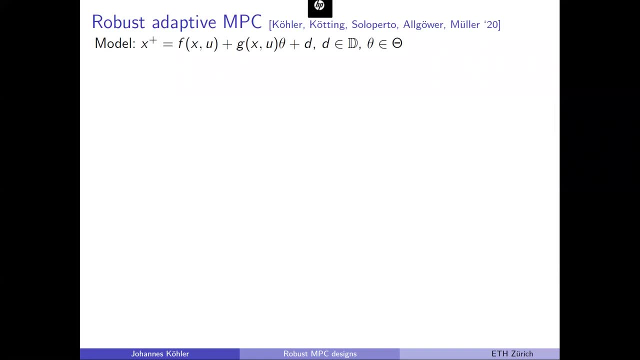 in any case. So, first, regarding the online model adaptation, the most standard case would be to have a model of this form In any case. In any case, where we have a known model, where we have a known model, We have a known model in India and another parameter and some additive disturbances. 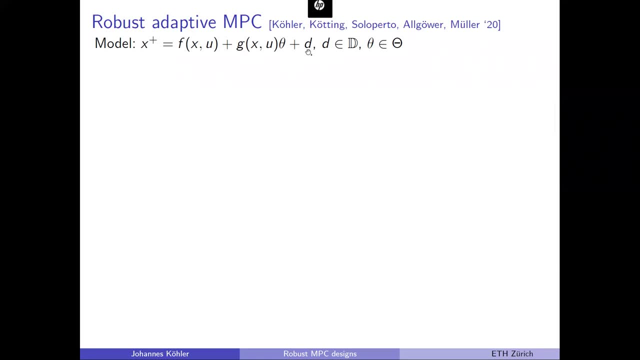 We have a known model. We have a known model in India and another parameter For this. the first thing you can do is called set membership estimation. The first thing you can do is called set membership estimation, So we can use the knowledge of the maximum austerity versus. 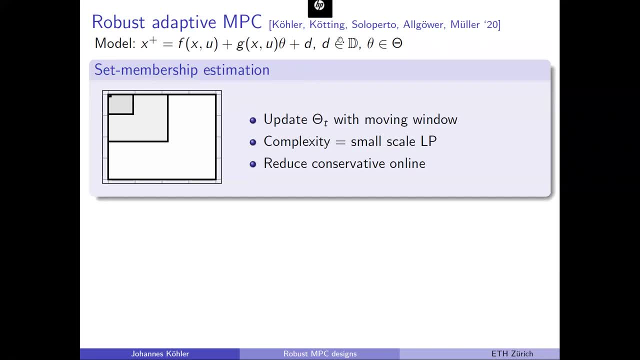 and past-date input measurements to determine this set of And past-date input measurements to determine this set of allocations. to get a elves and an adapter: pre-orbiter aspect average: the set of all possible parameters consistent with the data. Then by using a moving window approach. 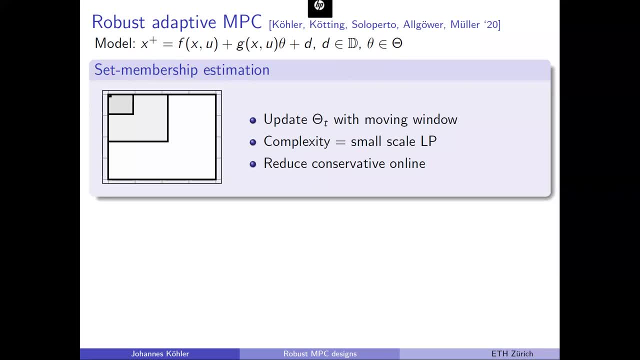 where we process multiple data from the past in one go and a fixed parameterization. for example, here, by given by a box, you can online compute shrinking boxes which contain the true parameter and thus reduce the conservatism online. What's important, at least in the case of 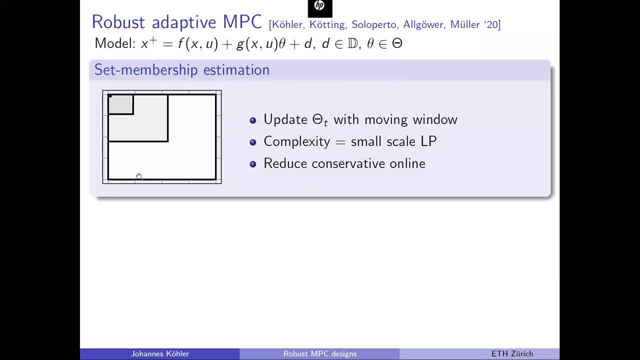 polytopic disturbances. this whole updated procedure only requires the solution of small scale in your program, so rather less liberal computational demand. In addition to the set membership estimation, we can also use adaptation for stability, particularly if we use a least mean square point estimate and define a new trajectory based on this point. 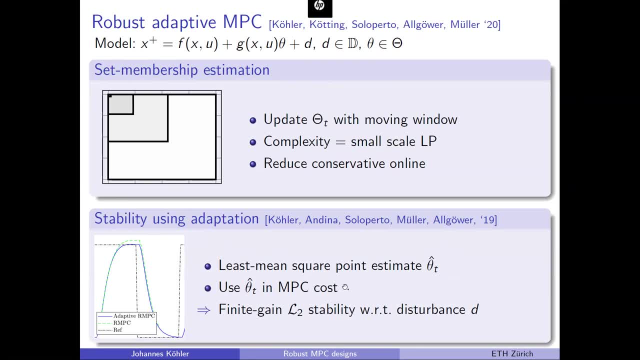 estimator and use this in the cost function in MPC. then, under some additional conditions regarding cost, under reduced need, performance and so on- mainly quadratic costs- we can ensure finite gain L2 stability with respect to disturbances. So this particular means if there are no disturbances. 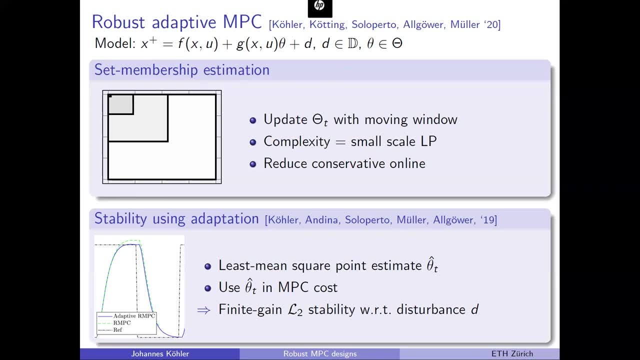 but initial parameter error, we can still guarantee that we will asymptotically converge to the correct steady state, And we can see the effect of this here. on the left, There we have a robust MPC formulation which is safe but results in some offset, while we have also 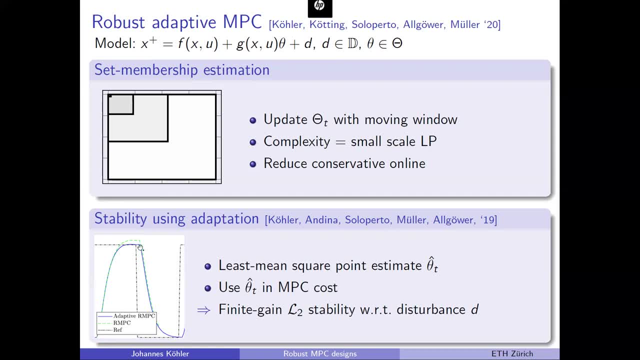 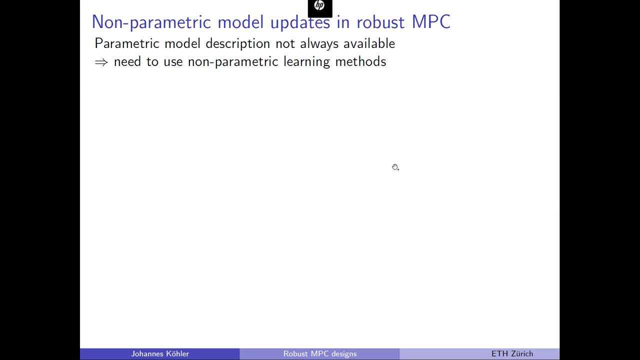 robust adaptive formulation which converges faster into the correct steady state. So this is all for parametric models. Sometimes, while we do not want to use parametric models, we cannot use parametric models. In this case, we have to resort to non-parametric models. 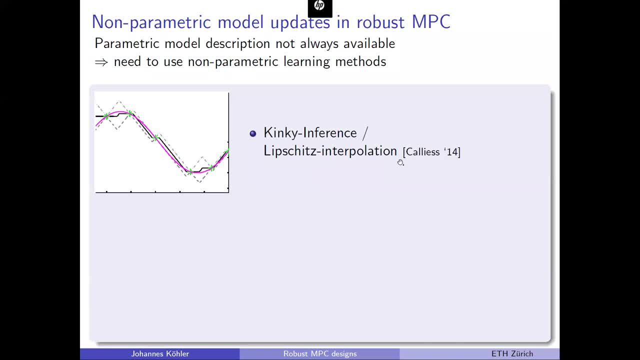 There are largely two classes of non-parametric models: One, Kinky inference, also called Lipschitz interpolation- They use a known Lipschitz model on a system to determine a set of possible functions characterizing our system- And the other is kernel-based regression. 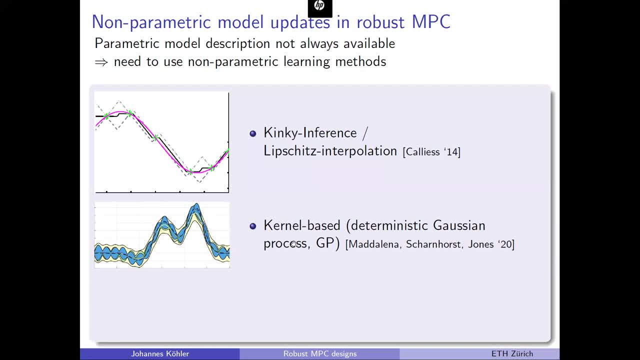 like deterministic Gaussian processes And what's important for both of those systems, if we do non-parametric model updates. there are some conditions under which, for both Kinky inference and kernel-based methods, there may be some more restrictive conditions. You can find uncertainty characterizations. 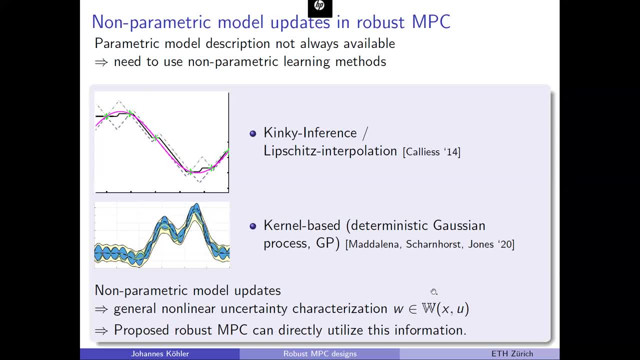 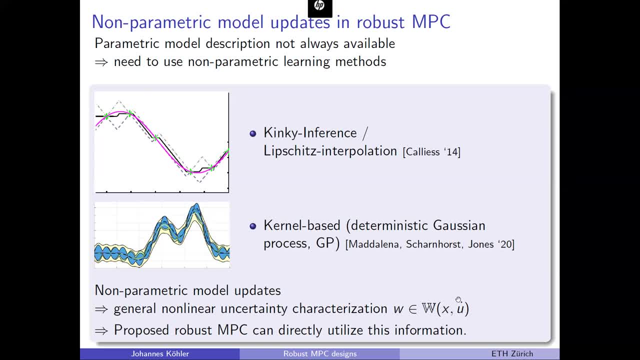 in dependence of the state and input. Another main point I want to point out here is that, even though those expressions are very nonlinear, they can be directly incorporated in the robust MPC approach I showed you before where we can incorporate general static bounds on model mismatch. 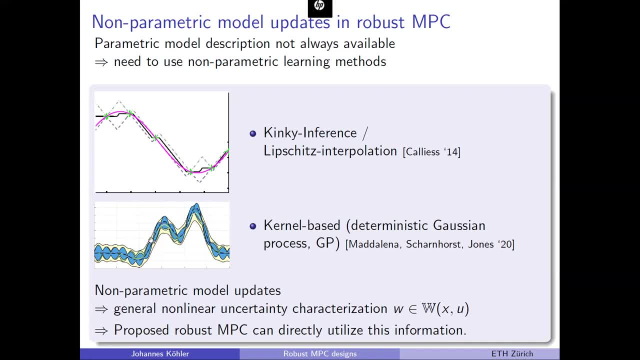 So for example here, this knowledge how large the model mismatch is at different points in state space can be incorporated in the MPC approach. So this may be a major reason why we want to use this model of MATLAB to help the MPC design track more cautiously. 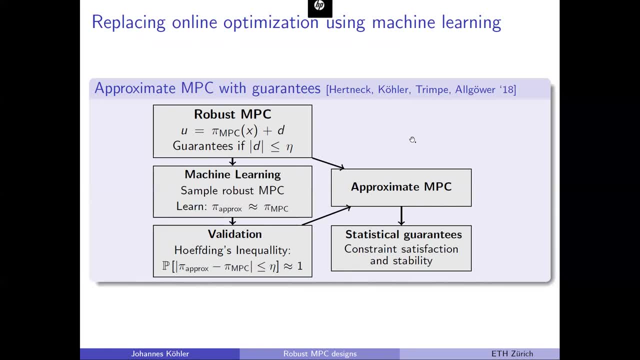 and avoid unsafe regions. Now the other thing I want to briefly discuss now, which is not model adaptation, but to get rid of the online computation completely. So the reason why this might be interesting is that we often, even though the optimization time 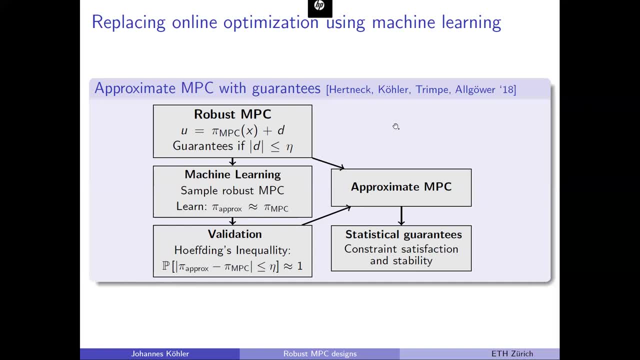 is one of the most critical points and if we can get rid of it completely, similar often allows for simple implementation, and one conceptual way to do this is sketched here, where we start by designing a robust npc formulation. then we use machine learning techniques to approximate this implicit multiplicative control law, for example by 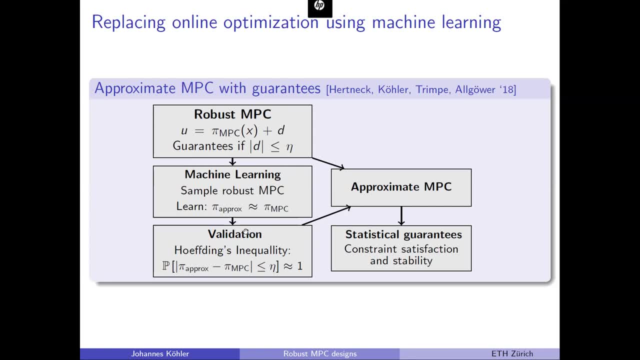 neural network controller. then we use validation to ensure that the difference between the original robust npc and this neural network controller is small, and then, by combining the robustness properties with the small approximation arrow, we get an approximate npc in the term of a neural network controller which still shares the same theoretical properties regarding constraint. 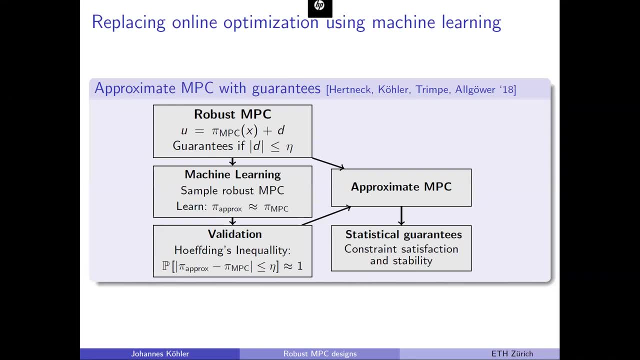 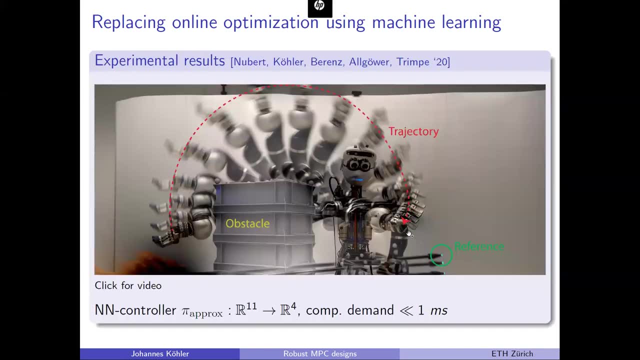 satisfaction and stability. so now we only have to implement a neural network controller, but still keeping most of our theoretical guarantees. and this is a recent experimental result for this robotic manipulator- where we're able to actually show that this works for real systems. and here we have. 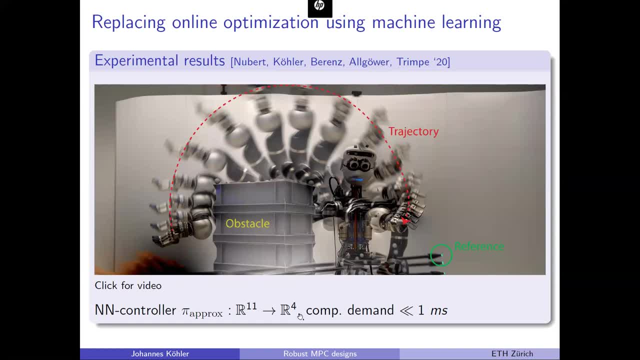 an 11 dimensional parameter vector which maps to four dimensional inputs to solve this tracking problem and we approximate this overall npc which solves tracking, inverse kinematics and everything with a neural network and actually evaluating this is no problem, in less than one millisecond, even on cheap hardware. and just to give you an idea of the fast sampling times we can achieve: 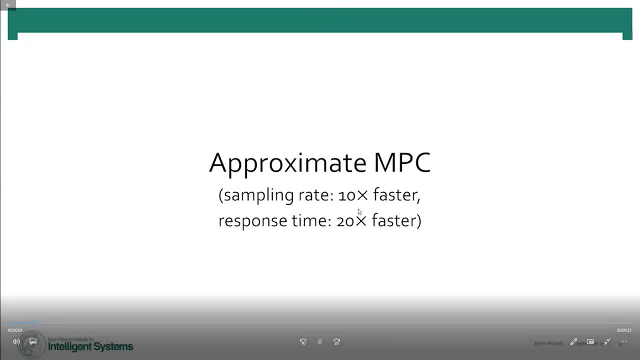 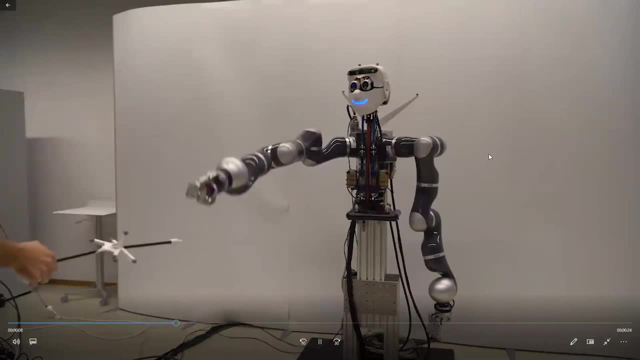 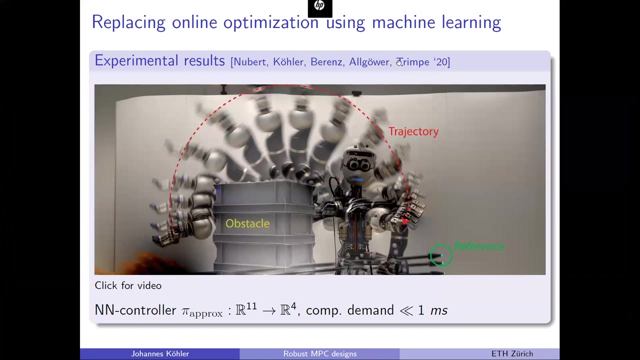 with this and quick reaction. i have a brief video here, but this is what it looks like in real time. so here the robot has to track this stick given from motion capture. okay, yeah, and so this works. it's also applicable to real systems and you can really implement it. 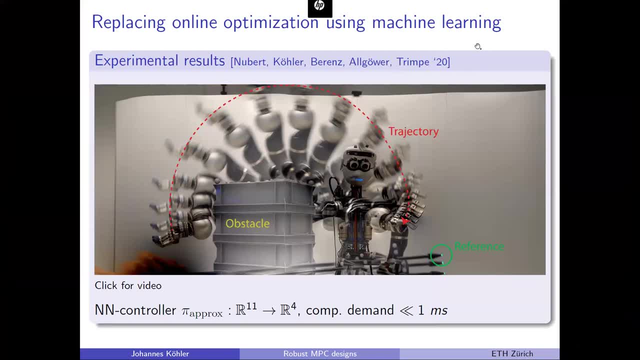 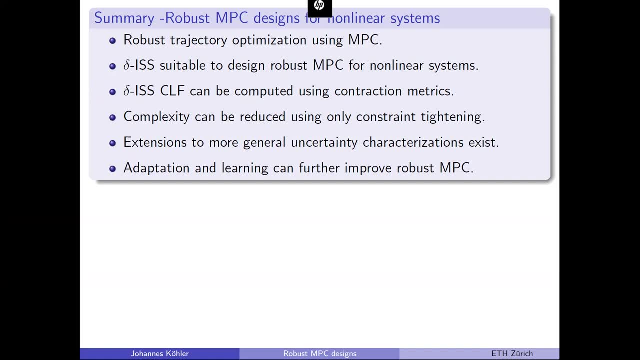 but it has more offline demand for the sign. Okay, with this, I'm at the summary of my talk. We looked at robust trajectory optimization using model predictive control. First, I would argue that incremental stability is the right tool to look at robust uncertainty propagation. 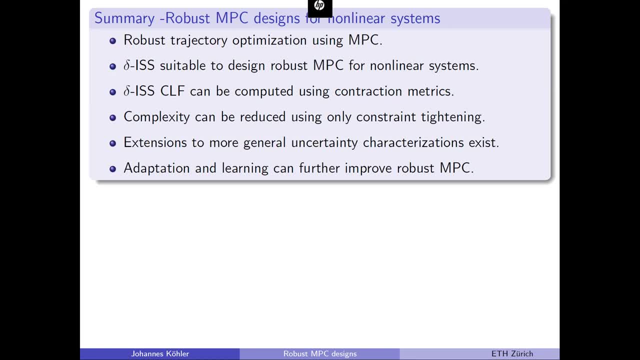 for nonlinear systems and thus for robust MPC-designed nonlinear systems. I showed how corresponding incremental YAPL functions can be computed using contraction matrices. Then I showed how we can reduce the computational demand of the MPC to equivalent to a normal MPC by only using constraint tightening. 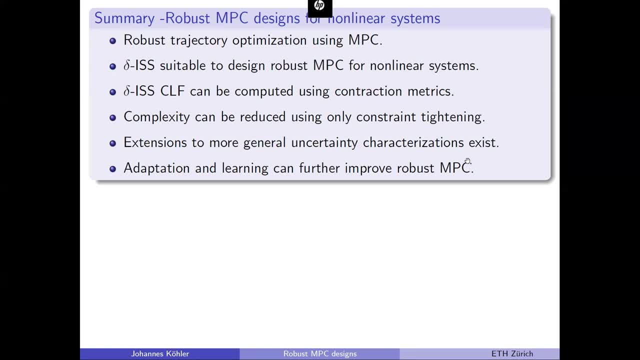 We discussed how more general uncertainty characterizations instead of additive distances can yield better results. And, lastly, I briefly mentioned how adaptation and learning can further improve robust MPC. Before I end my talk, I want to briefly mention some collaborators with whom I worked on those results. 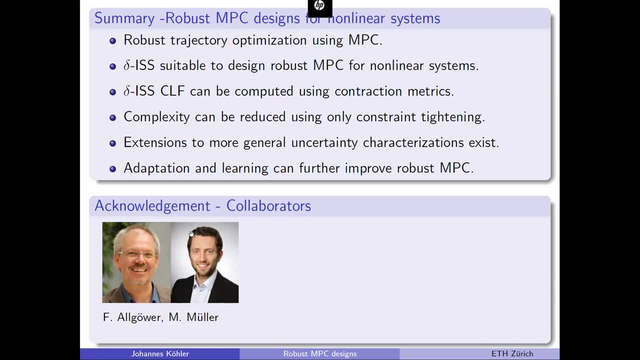 First my former PhD advisor Frank Agarwal from Stanford, and then my former PhD advisor Frank Agarwal from Stanford, and then my former PhD advisor Frank Agarwal from Stanford and Matthias Müller from Hannover, with whom I derived most of the results I presented today. 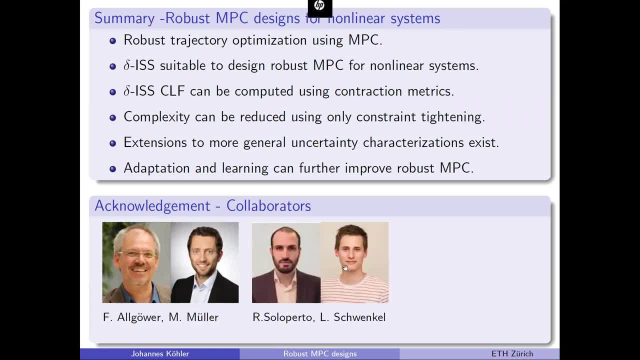 My former colleagues Rafael S Loperto and Lukas Schwenkel from Stuttgart, with whom I developed the robust adaptive MPC and dynamic uncertainties in MPC, and also static uncertainty bounds in robust MPC, And also Sebastian Trimpe from Aachen and Julian Neubert. 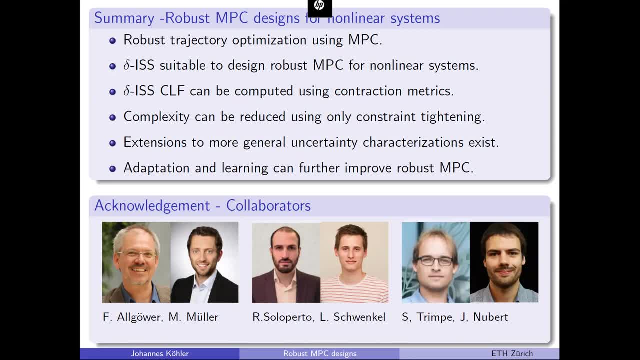 who is now a PhD student at ETH, who did this approximation of MPC using neural networks and also the robotics implementations. In addition, I want to acknowledge some students who helped further: Michal Heltnig, who had some initial contributions for the approximations. 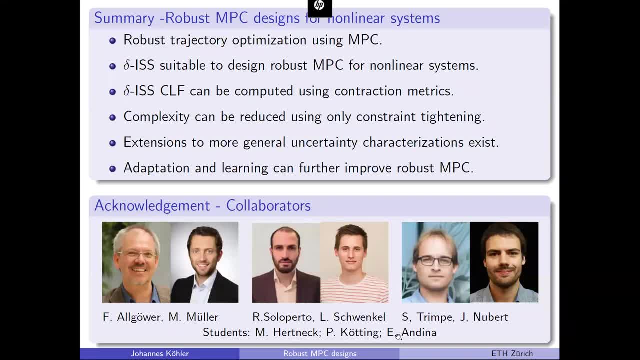 of MPC schemes, and Peter Kurting and Elisa and Dina who worked on adaptive MPC. With this, I'm at the end of my talk and I'll be very happy to answer your questions. Thank you, Ioannis, for the great talk. 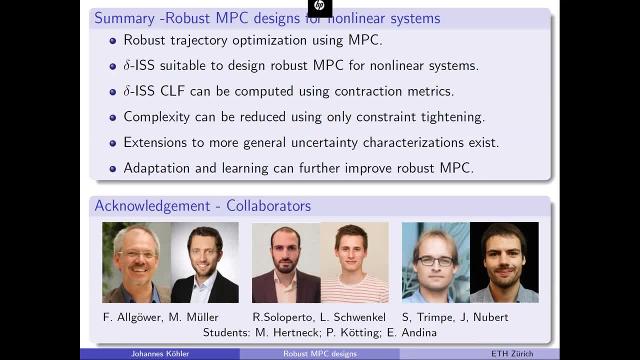 Are there any questions from the audience? I have one question Go ahead. So thanks for the nice presentation. So the controller that you designed actually needs to be robust against the whole range of the disturbance, And this is somehow conservative because maybe there is no feasible solution for that. 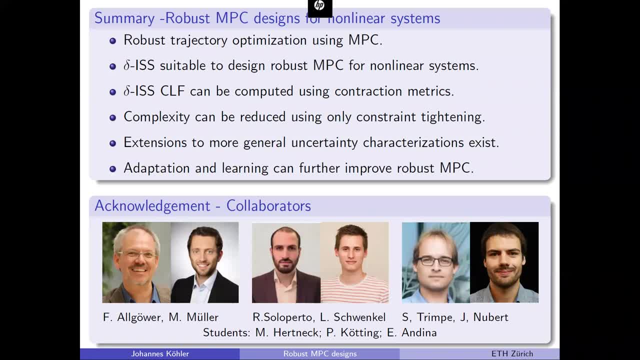 So isn't it better to assign some distribution to the uncertainty disturbance here and go for a stochastic version of this delta ISS property and to provide some sort of probabilistic guarantee? Now you have solution using this approach, but this is not for sure. 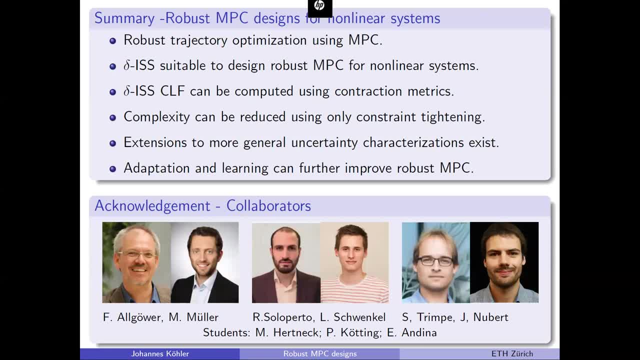 There are some probability behind the solution, But at least we have some actually kind of solution for that. Just we need to provide the stochastic version of this delta ISS. What do you think This is not actually less conservative and more realistic approach? So first let me agree. 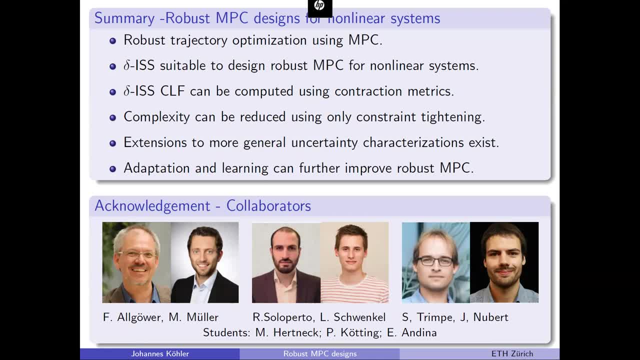 Yeah, in general, robust control in general and thus also robust MPC, is more conservative than stochastic approaches, I would say right now, in my opinion, mostly stochastic is one step more complex than robust, And robust is not yet fully solved for those systems. 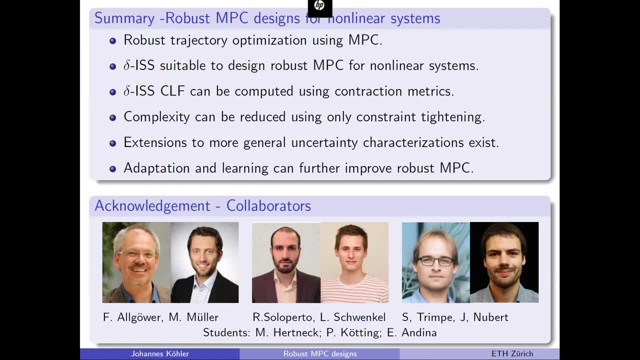 So it's a rather new topic- how to really do good robust predictions for systems at least cheaply implementable, And that's why I think it's important for the future to also look at stochastic. But it's not. There's still some work to be done to go there, I think. 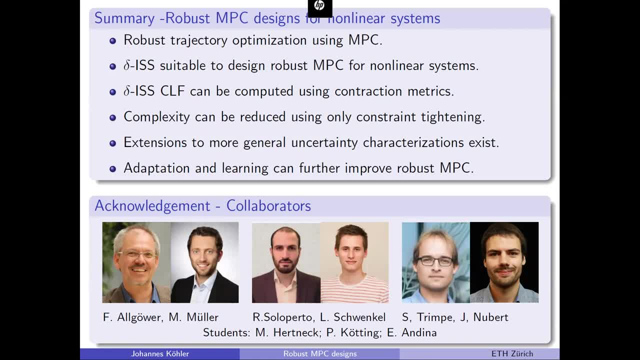 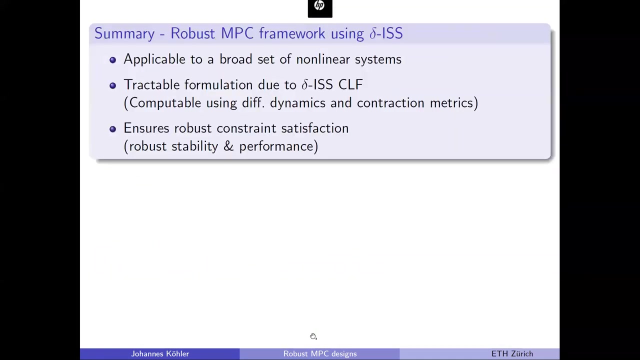 OK, OK, OK, thank you. Other questions: I've got a question to Dacus. Yeah, go ahead. So have you tried this also? for example, at the introduction you had this car maneuver- sort of lane cross, I think- example where you have other participants. 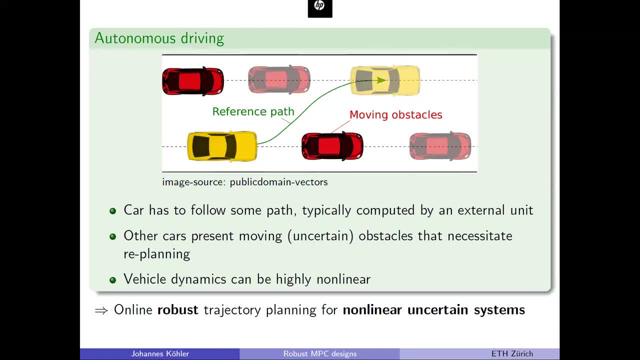 We have tried this out on such an example, So we have numerical implementations for this in the sense that. so if you have other participants and you want to stay in this kind of robust MPC thinking, what you typically assume or the way we did it, 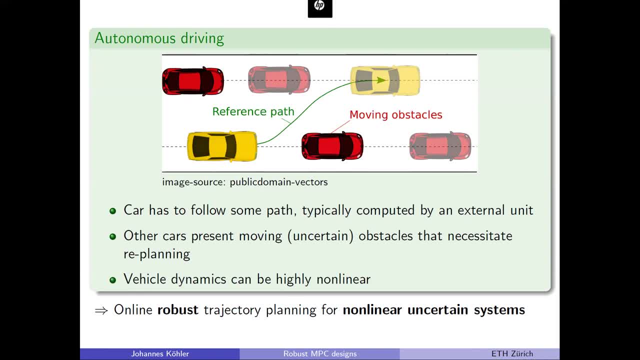 and then you can do this is that first you assume you know exactly what the other cars will do And then next you assume they only deviate by a certain amount in every time step from the previous pass. And if you have such assumptions, which for example, 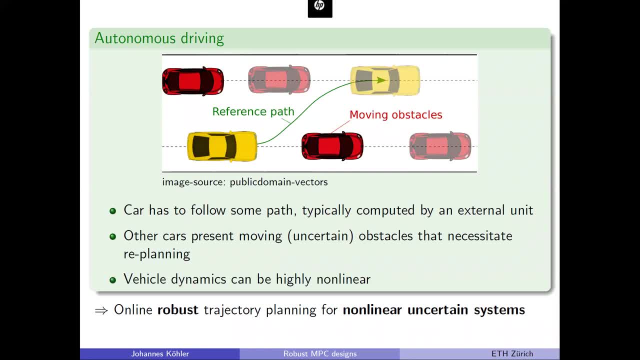 does not allow for drastic changes, but they can slow down a little bit. but we also had implementations where they can really break full and that's something you can incorporate. You will get more conservative, but that's actually numerically. at least we were able to implement it. 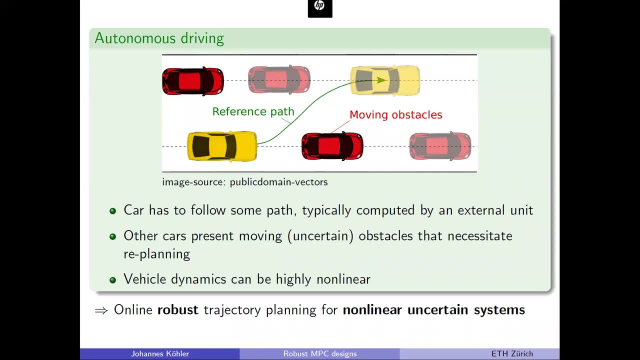 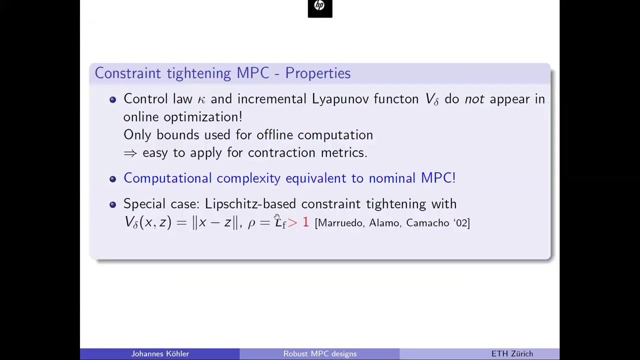 Thanks, All right, It seems there is another question. Maybe, Yeah, If we still have one minute. Yeah, Yeah, Yeah Yeah. I was quite curious about the computational gains with respect to the last example you showed. So you said you were able to approximate the MPC controller using a neural network. 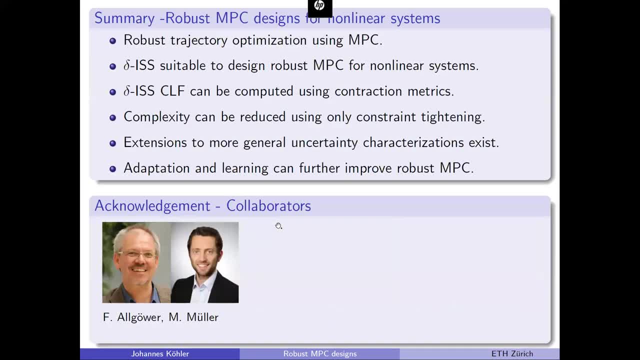 But I think I missed what was the original computational burden associated with it, The MPC controller. I'm not sure if I know it by heart. So I think we're first If we solve to full optimality, which we did for the same thing using Cassadis or nothing. 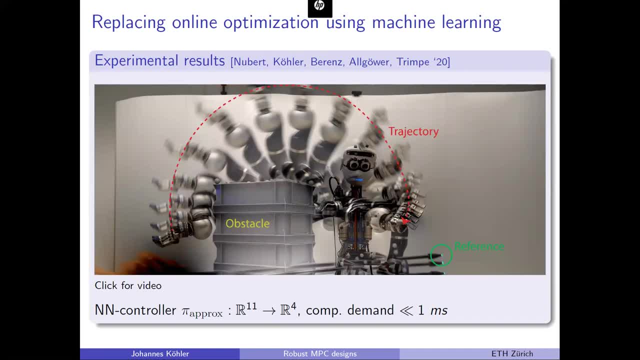 tailored. Yeah, I think it can do it a lot better. It was 400 milliseconds, So I think if you do real time, you can do a lot faster. Okay, But my main point would be the neural network. It's not that, it's now one millisecond. 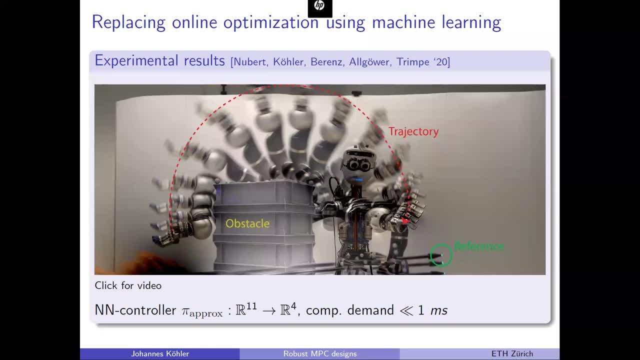